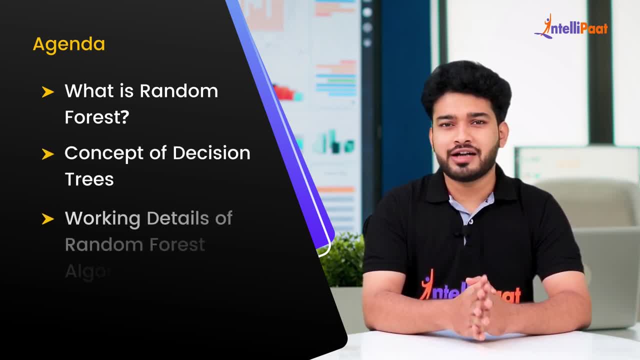 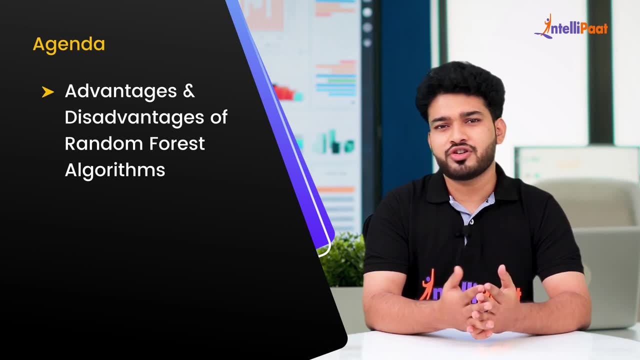 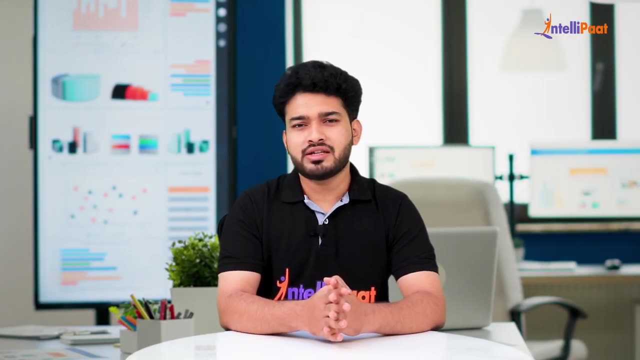 of decision trees. Next we'll cover working details of Random Forest algorithm. After done with that, we'll talk about different advantages and disadvantages of Random Forest algorithm And finally, we'll cover hands on demonstration for Random Forest algorithm. I hope I have made myself clear with the agenda, So, without wasting any time, let's begin with. 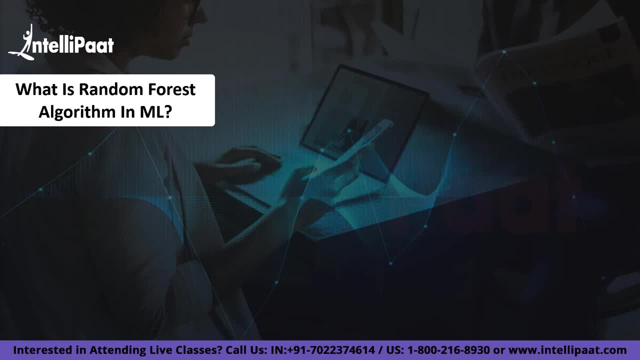 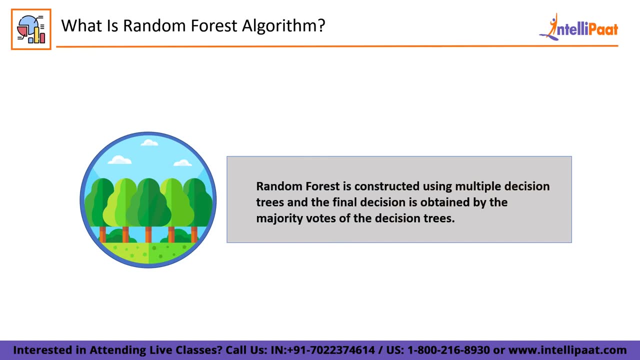 the first topic on our agenda. that is what exactly Random Forest is all about. So from the beginning, you can say that a Random Forest is something that groups multiple trees together and makes decision by putting intelligence gathered through these groupings to use. If 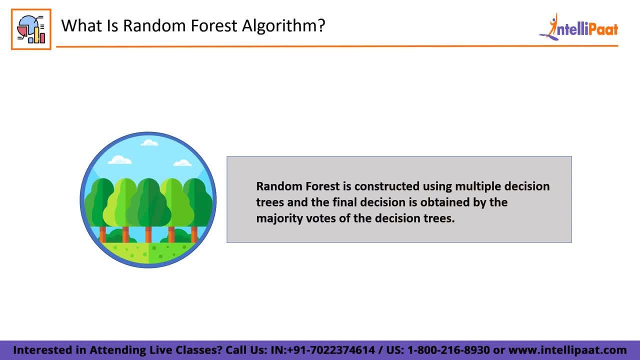 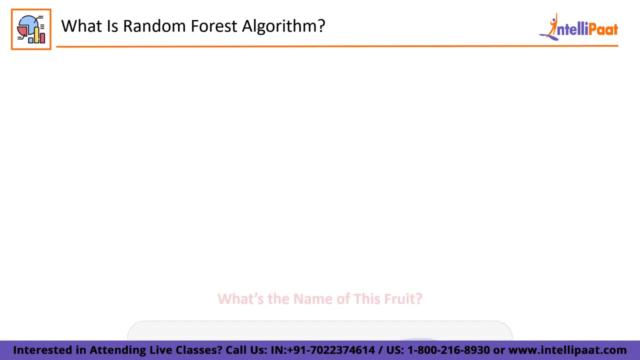 I had to formalize this definition, I'd say that the Random Forest algorithm groups multitude of decision trees together and then draws a decision based on the majority of votes these decision trees put forward. Let me make it more clear with the help of an example. 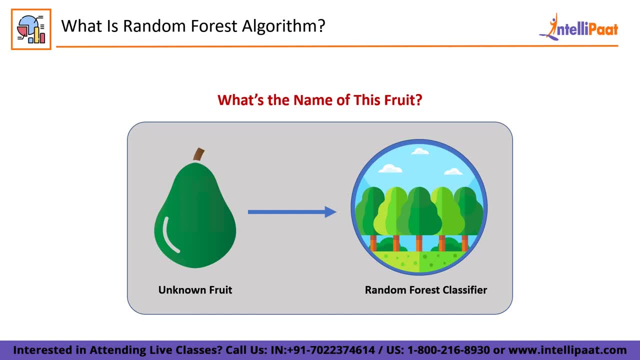 After that, we want to know the name of this particular fruit given over here and we ask this forest over here for help. Let's say, this forest here is a Random Forest algorithm and these trees that are part of this forest are decision trees. Now, when I ask this question, 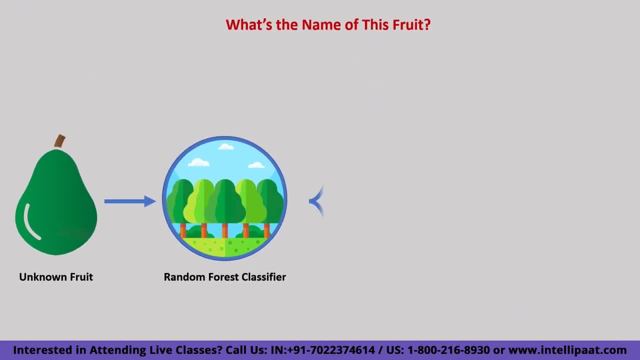 about fruit to this forest. what it does is it checks with the trees that are part of it. Another tree says that, according to me, this fruit is gava, And this third tree here- tree over here- says no, The tree one is right, This particular fruit is avocado. Now what? the? 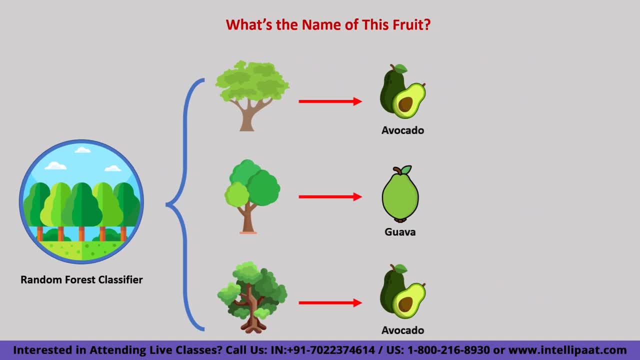 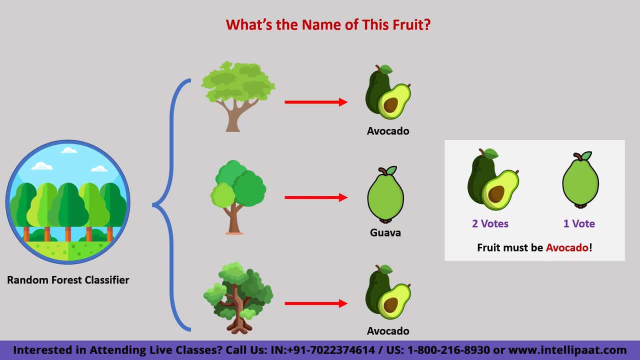 random forest does is: it takes the opinion of three trees and scores them Here. it says that I have two votes for avocado and one vote for gawa, So I think this fruit shall be avocado itself. So, basically, a random forest algorithm takes the decisions by utilizing learnings from multitude. 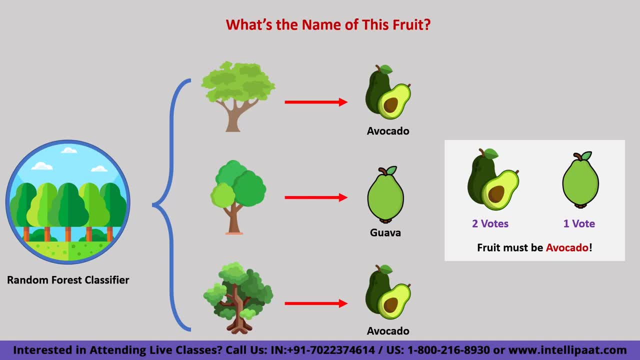 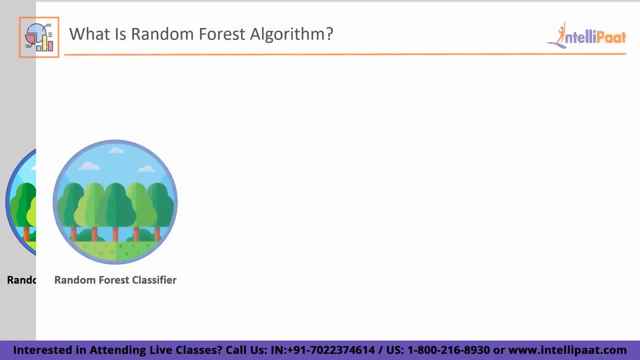 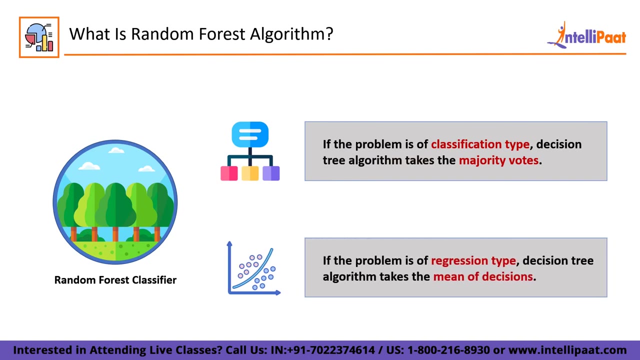 of decision trees and chooses the decision which has the maximum number of votes. Since this particular problem was a classification problem, the algorithm took the majority vote. Suppose if it was a regression problem, it would have taken the mean of decisions provided by trees. 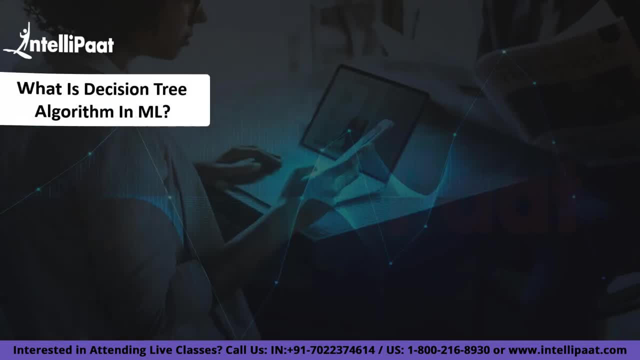 Now, that being said, let's first talk a little about the decision trees. So, guys, a decision tree is an algorithm used in machine learning which learns the relationship between data, attributes and labels to come across a decision. Now, if you are wondering how it is achieved, 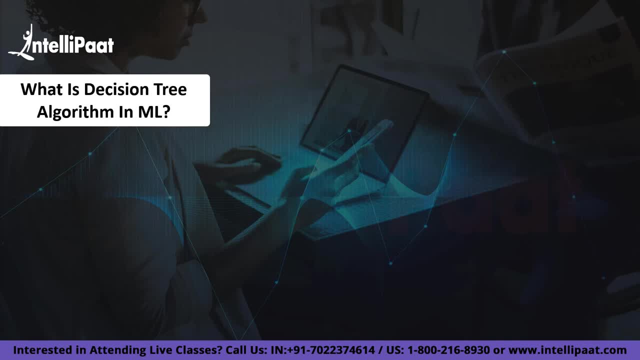 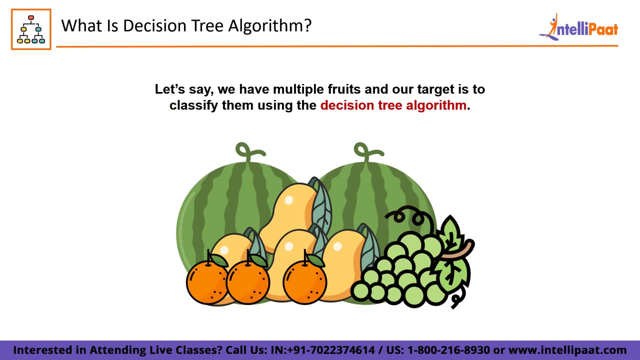 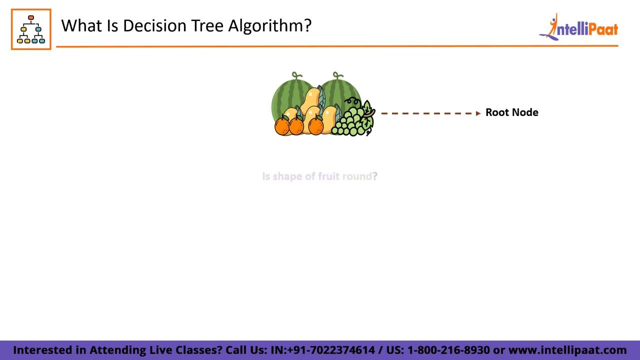 then let me explain that to you guys with an example. Let's say that I have multiple fruits over here and I want to classify them using the decision tree algorithm. Initially, all of these fruits will be kept at the root node. Then we'll put down the condition to split these fruits at. 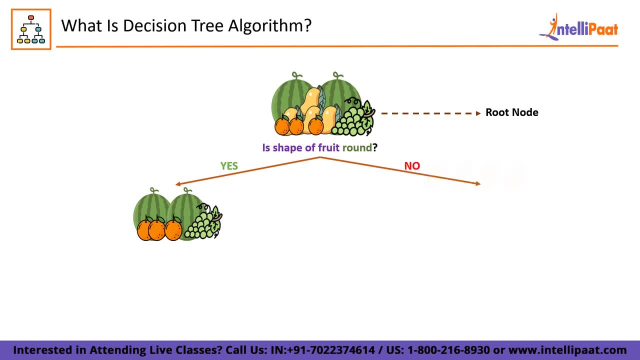 the next level. Now, let's say, we'll check whether the shape of the fruit is round or not. If it is round, it will go to the left side of the tree, and if it is not, then it will go to the right side of the tree. Now you can see that all the mangoes have been separated over here. Next, 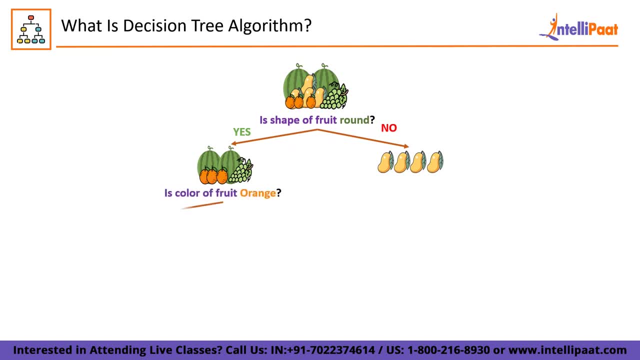 we'll just move ahead in the direction of the left node. Next condition will be to check whether the color is orange or not. With this condition, we'll have oranges separated from the lot Now. the next decision boundary we'll put across will be to check whether the diameter is greater than 10. 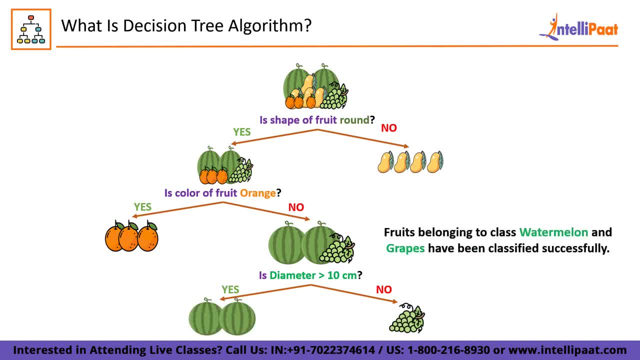 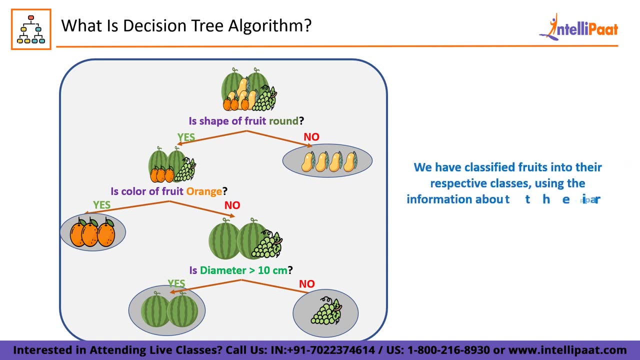 centimeter. If it is greater than 10 centimeter, the fruit will be watermelon and if not, the fruit will be grapes. Now, here you can observe that, with each node after the root node, we're actually classifying the data into its labels successfully, The last node, such as this node, representing 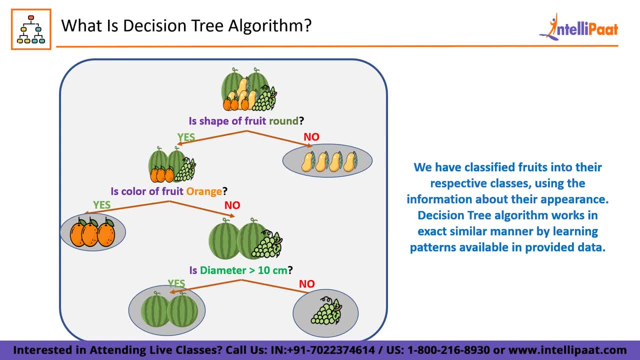 oranges, watermelons, mangoes and grapes are called as leaf nodes and- yes-no, decision boundaries you see over here are called as branches. I mean, this is just the minimum number of branches that are in the tree. So this is just a clear interpretation of how data can be used to make decisions in order. 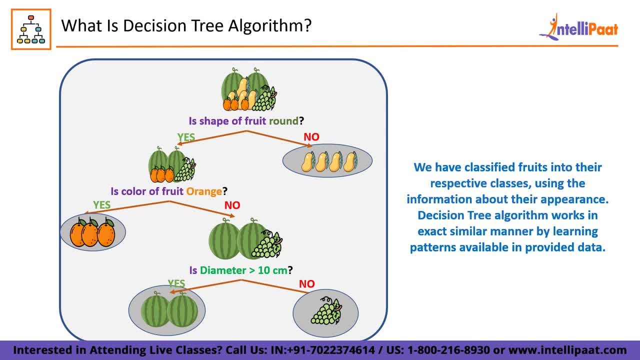 to classify the objects, But in reality, this algorithm uses multiple criteria, such as gene impurity, entropy and information gain. We have explained these criteria in detail in the previous video, where we covered the concept of decision trees. If you don't have a bright idea about, 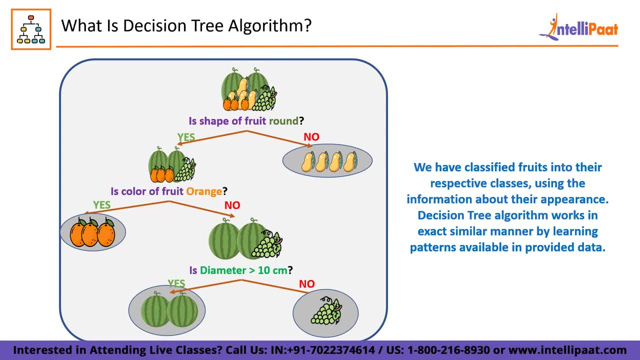 these statistical terms, then I would highly recommend you to check that video. You can find the getaway to that video in the description box, So let's get started. Alright, that being said, let's jump onto the next agenda pointer on our list, that is: 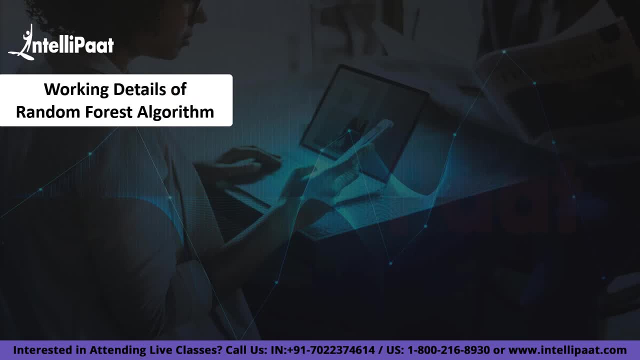 understanding the working details of random forest algorithm. In order to understand the random forest, there is set methodology that we'll have to follow. The process of this classifier begins by building the forest and ends up with making the prediction. So, first of all, let us try and 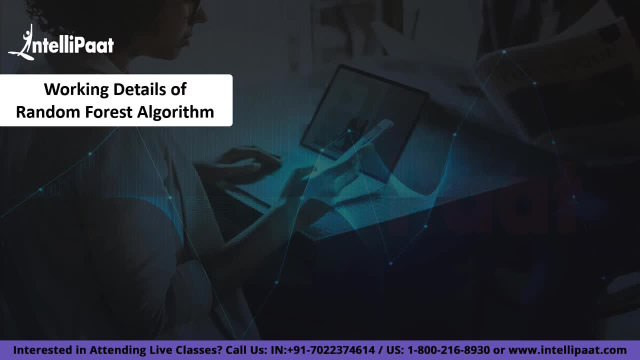 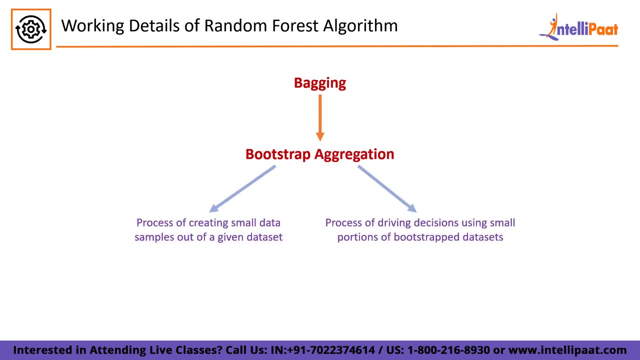 understand how the random forest algorithm works. So let's start with the prediction. The first thing we got to understand over here is bagging or bootstrap aggregation. So these terms incorporate two different procedures: bootstrapping and aggregation. Bootstrapping is the process of 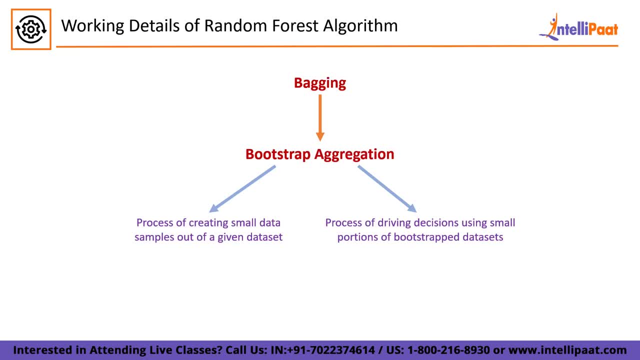 creating small data samples out of a given dataset, and aggregation is the process of driving decisions using small portions of bootstrap datasets. I know this is quite difficult to comprehend with just definition stuff, So let's start with bootstrapping and aggregation. So let's start with 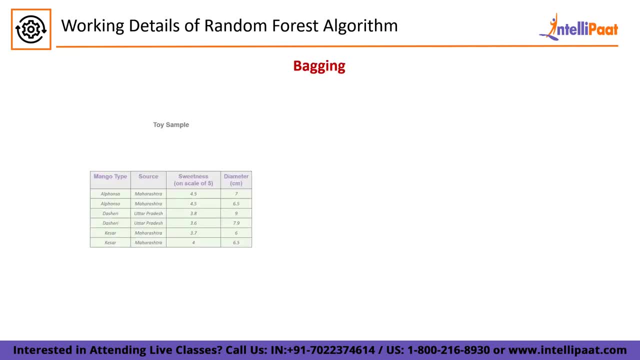 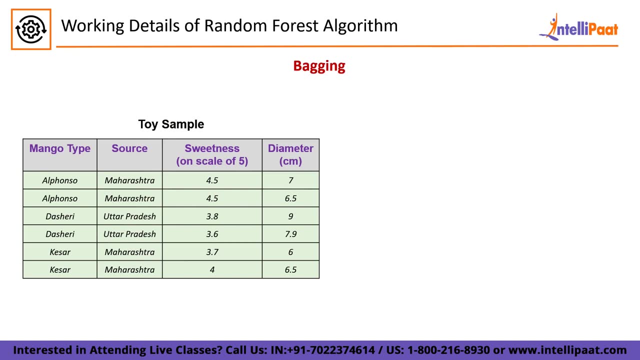 bootstrapping and aggregation. So let me put it forward with the help of an example. Consider this small portion of data over here. Basically, this is a toy sample that I have created to help you understand the working of random forest algorithm. This small sample of dataset covers: 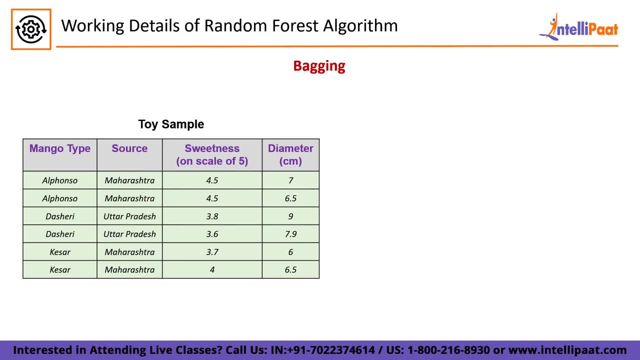 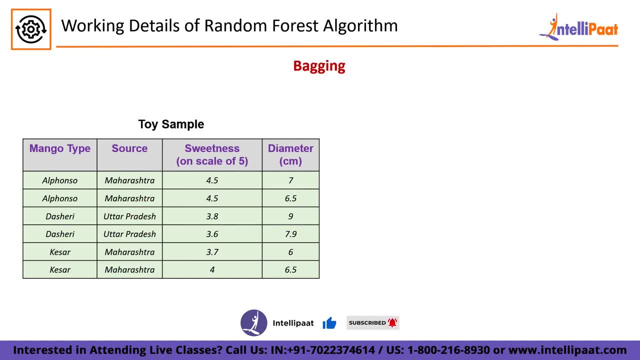 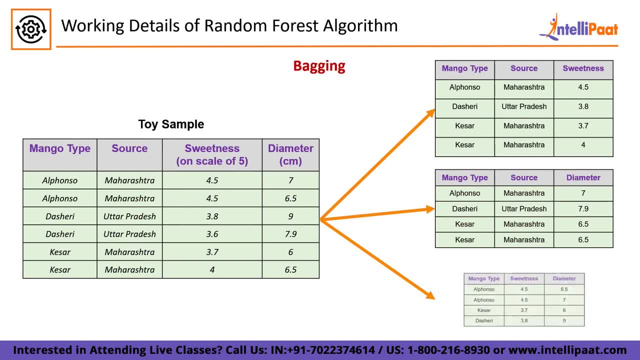 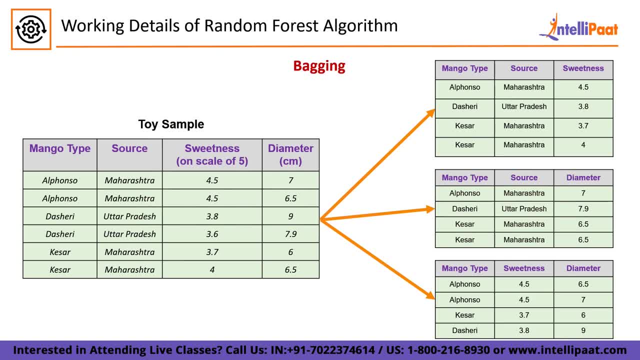 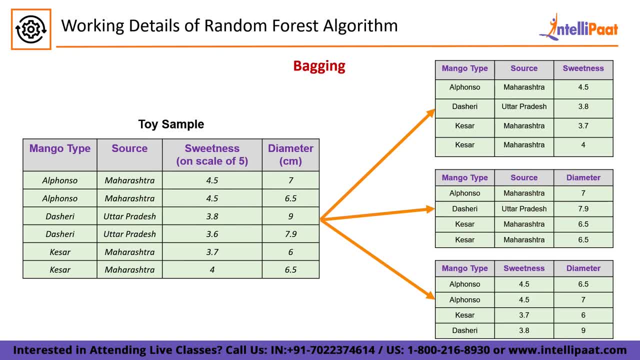 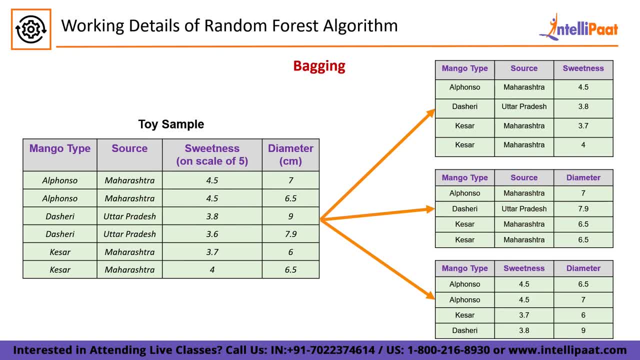 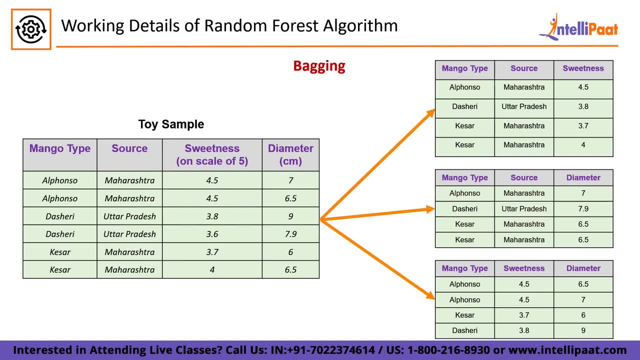 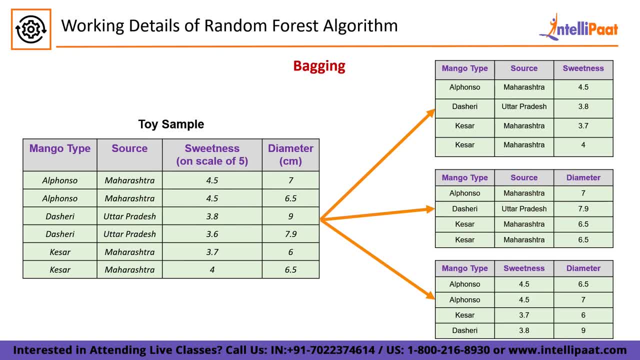 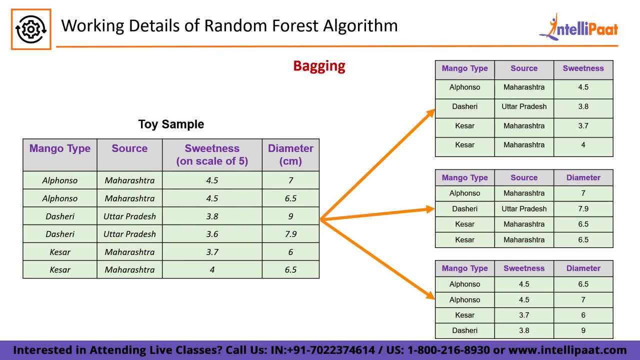 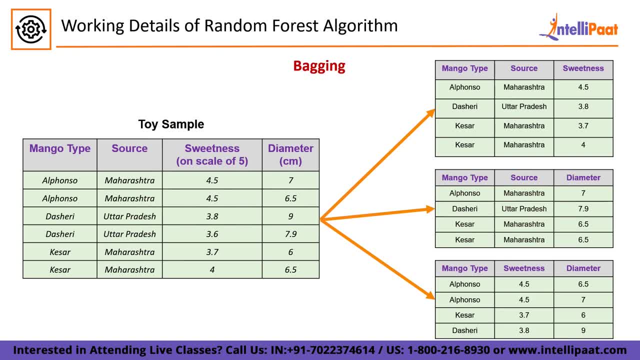 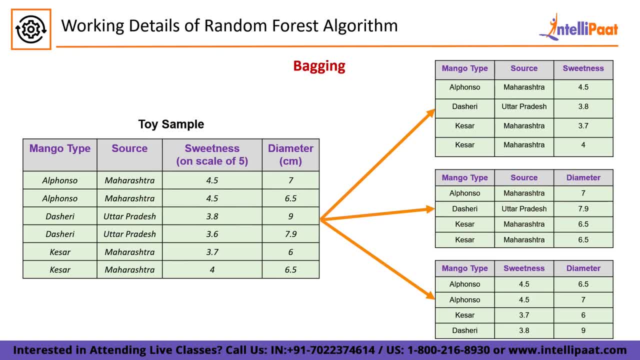 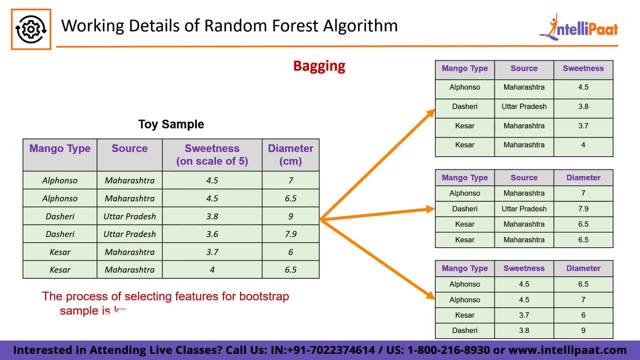 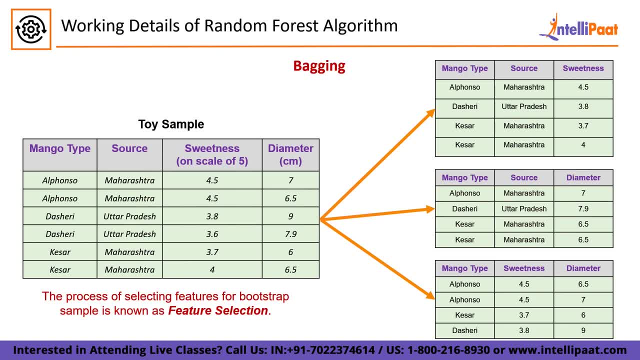 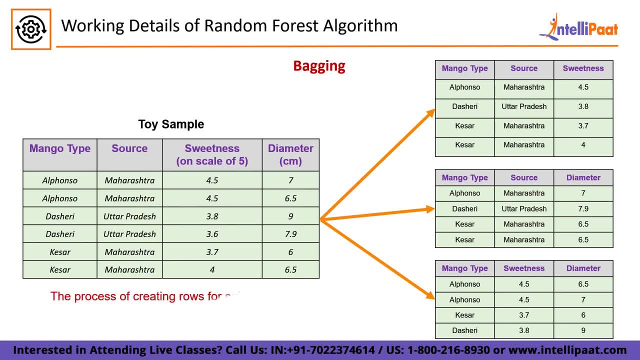 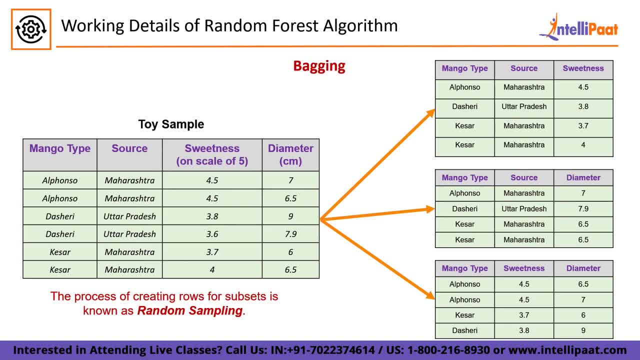 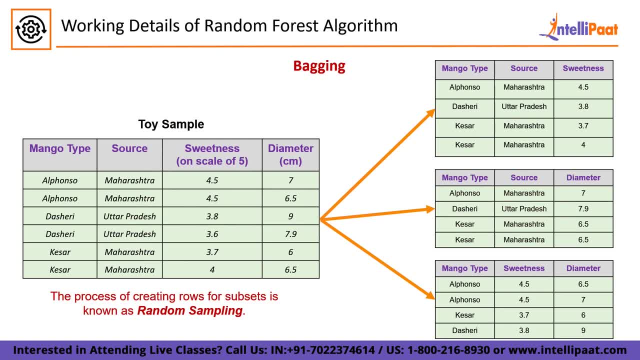 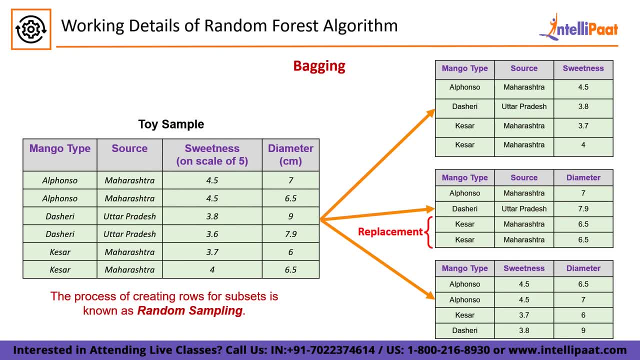 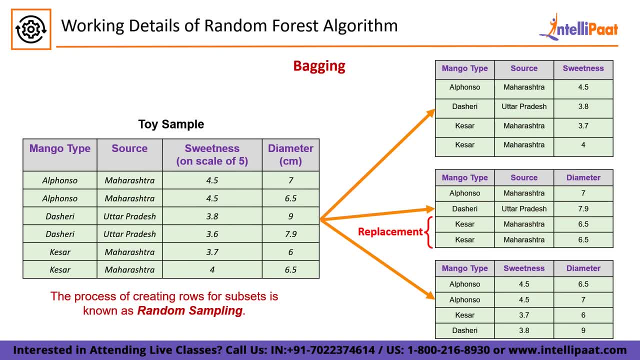 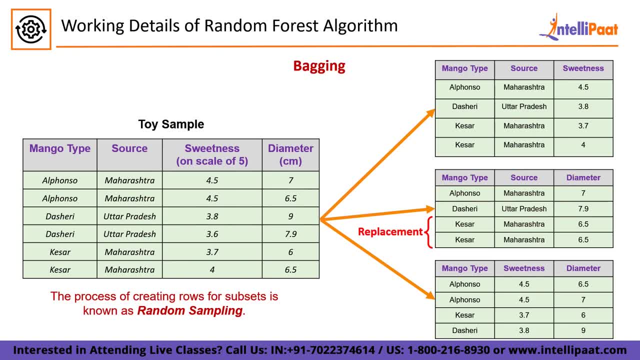 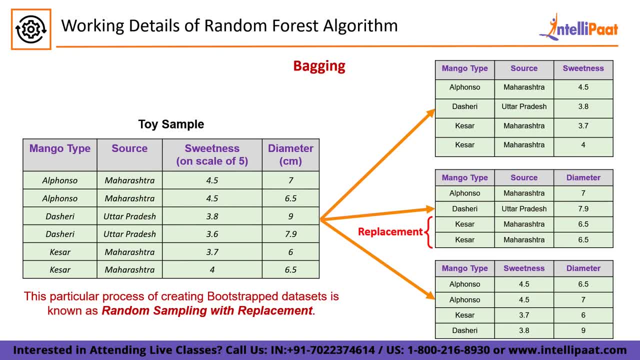 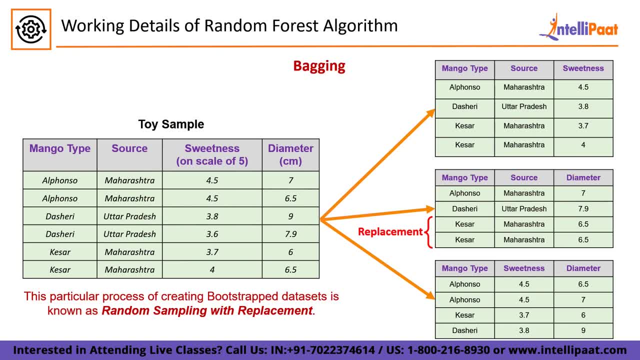 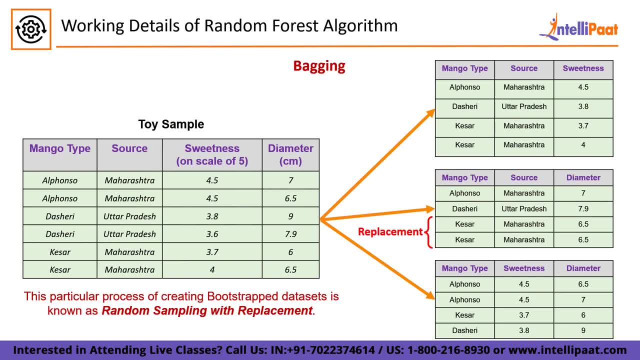 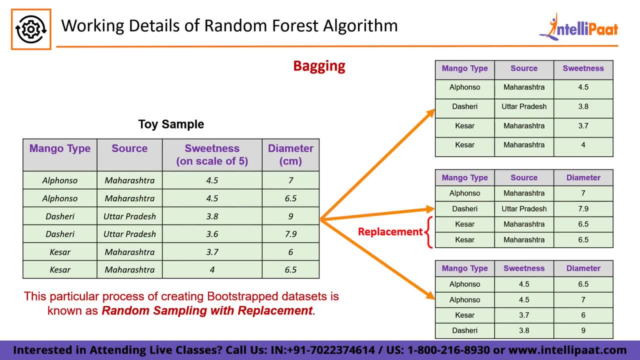 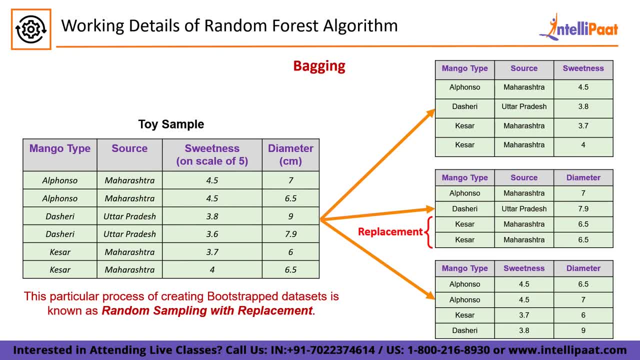 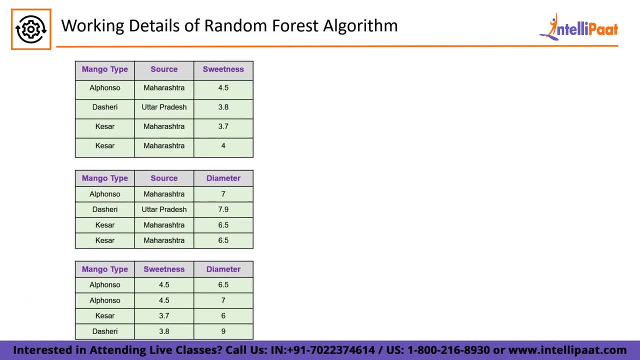 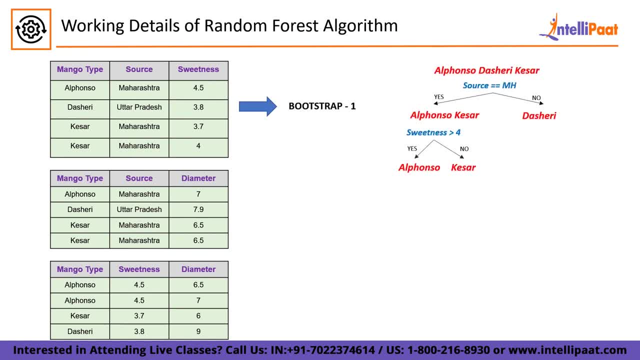 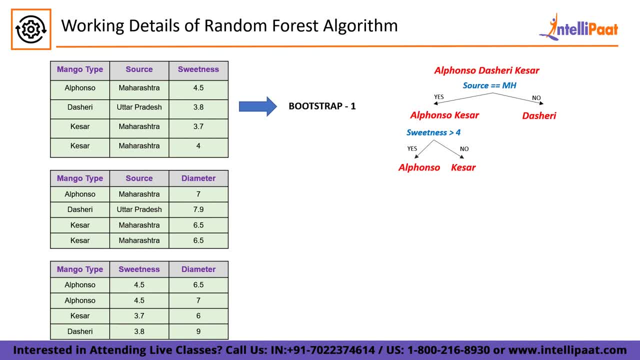 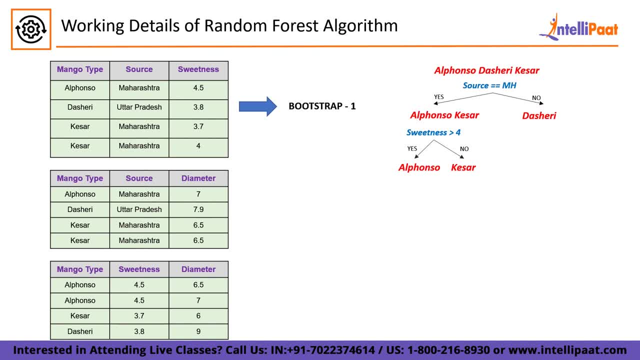 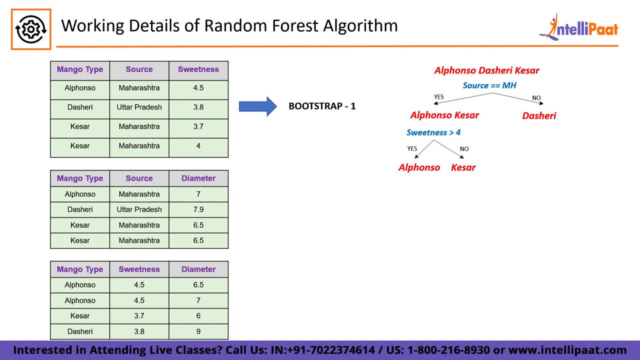 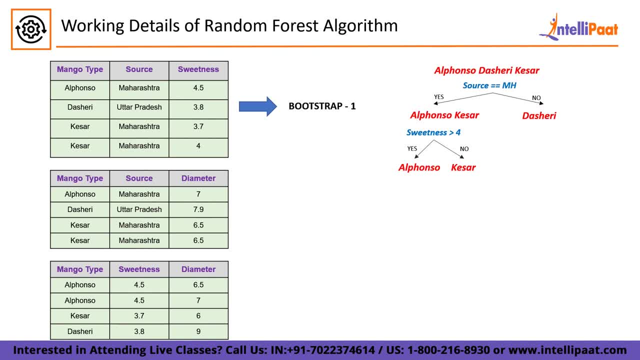 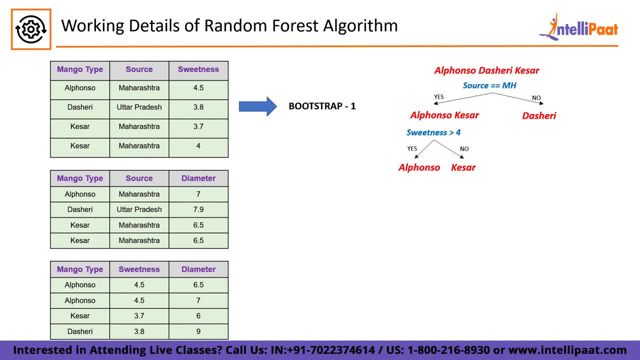 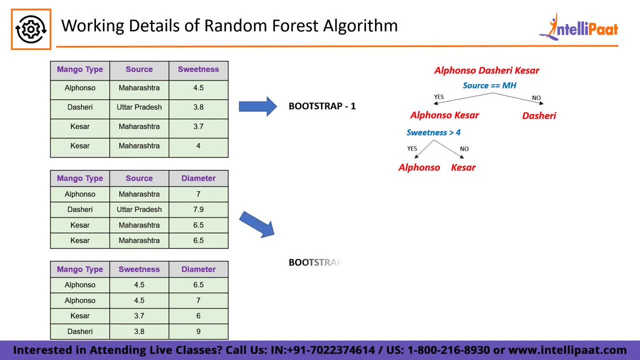 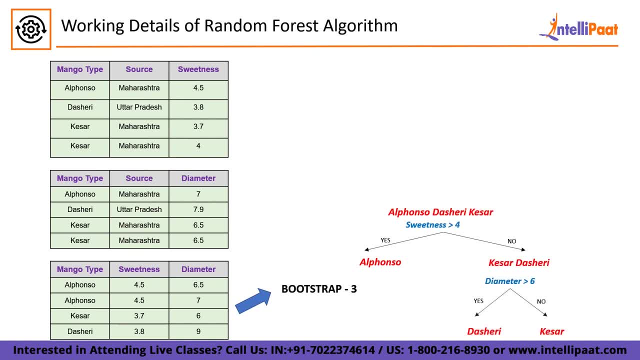 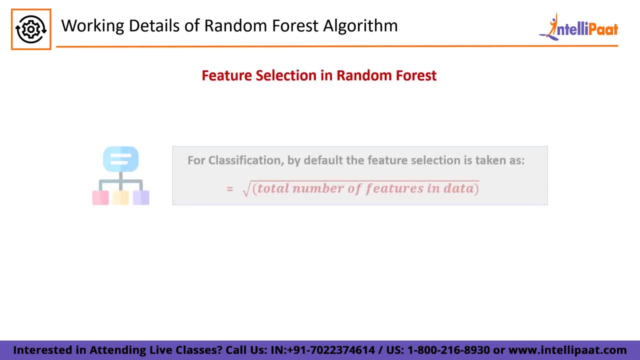 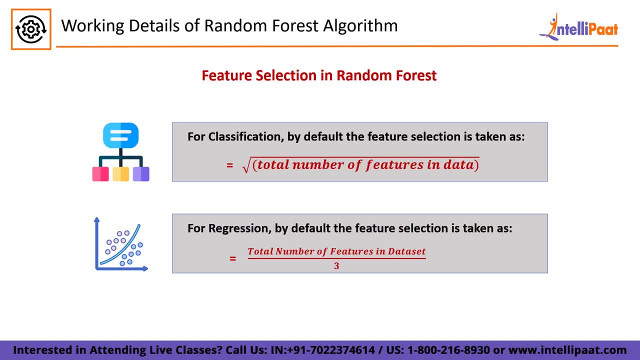 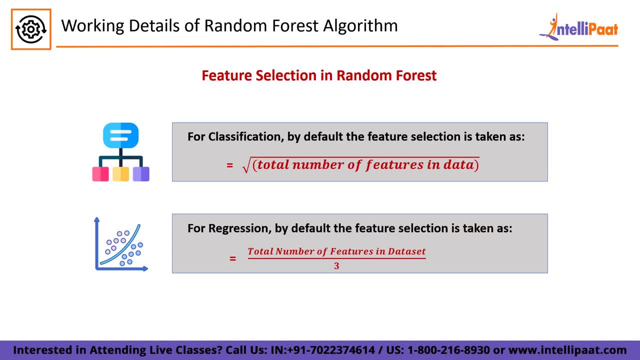 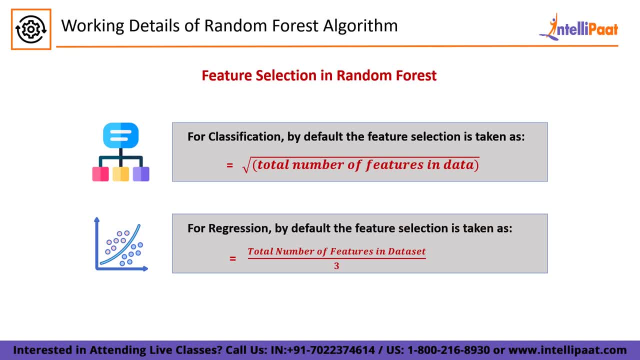 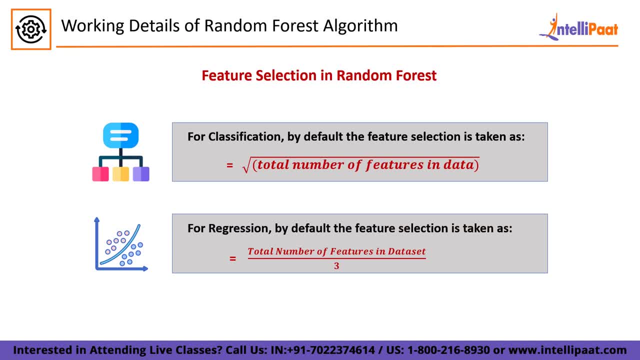 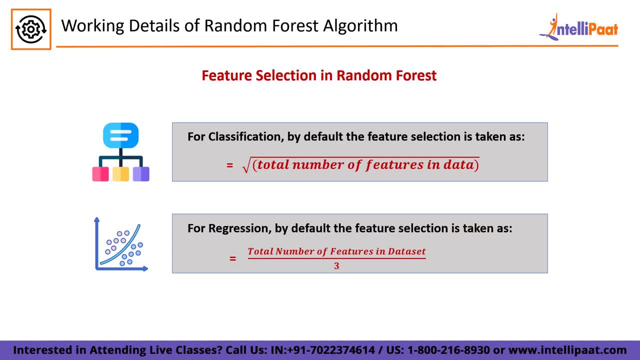 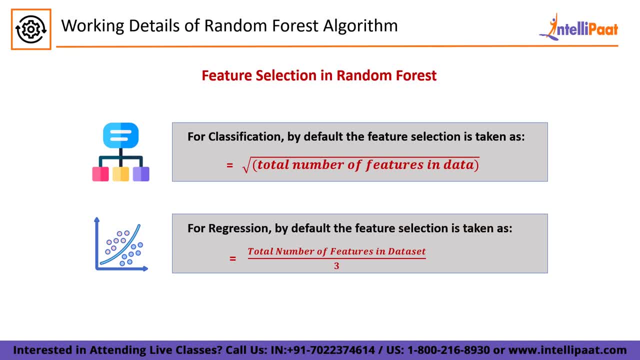 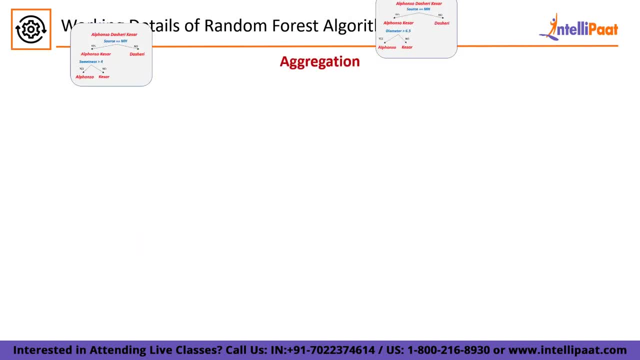 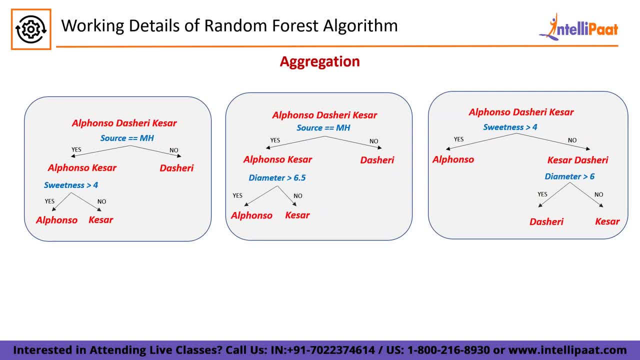 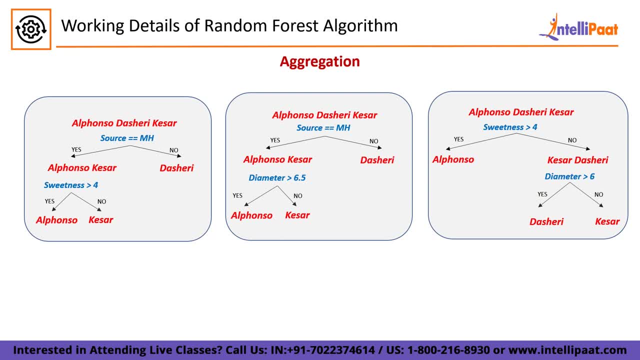 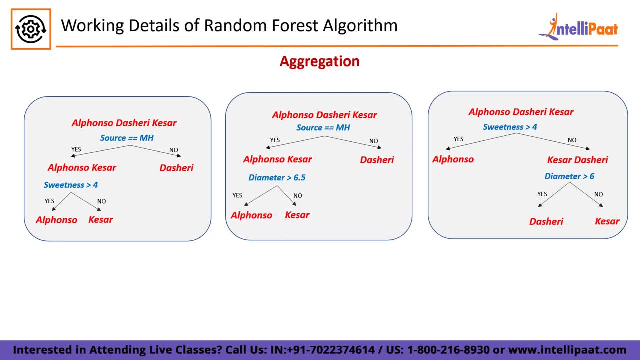 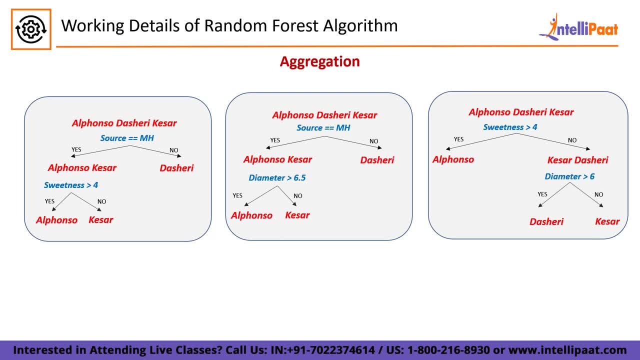 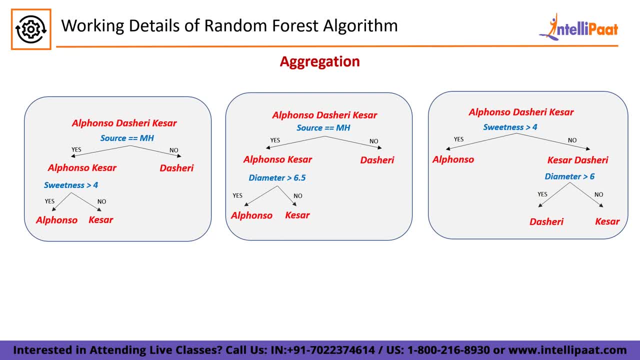 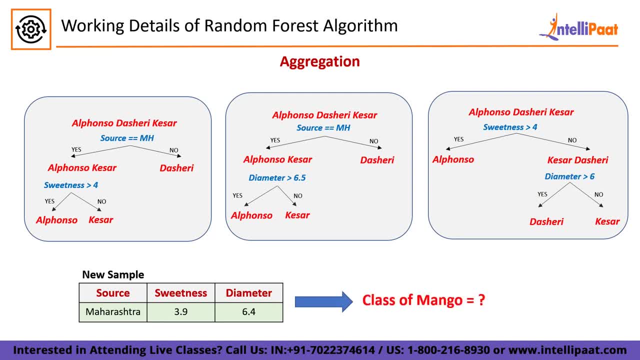 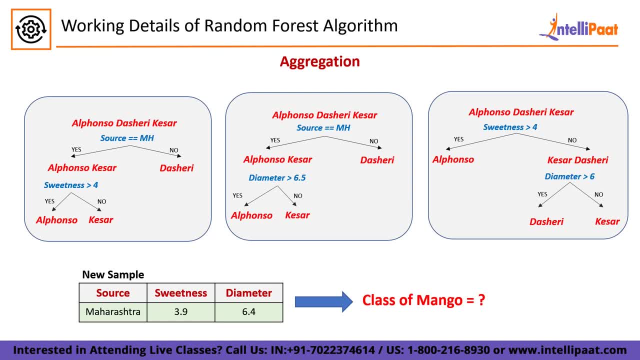 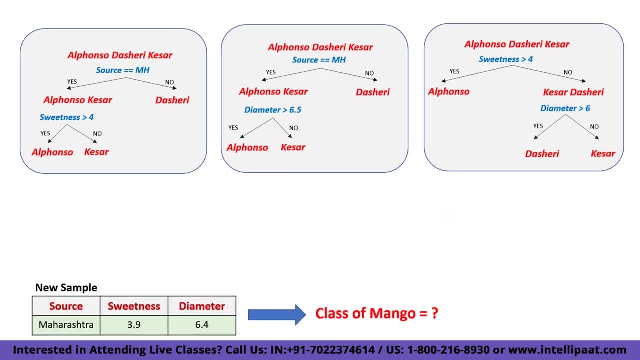 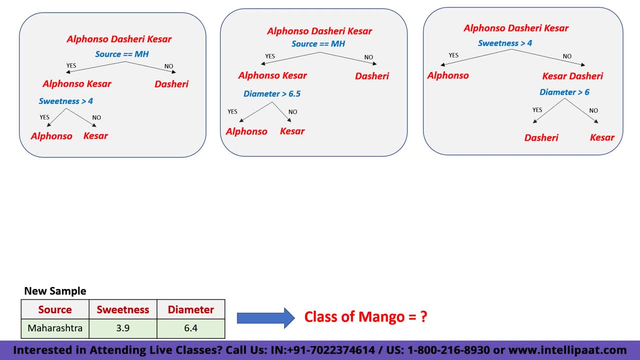 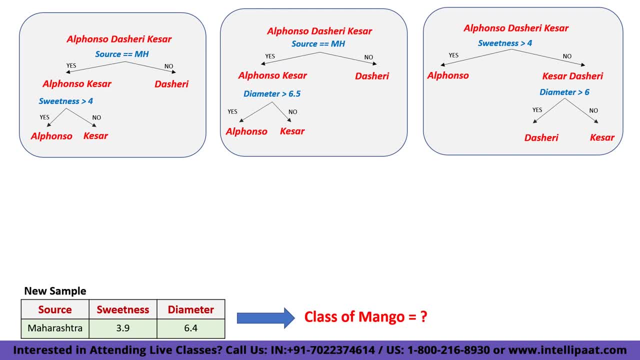 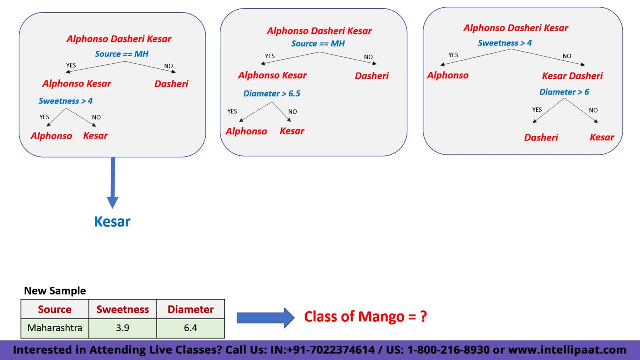 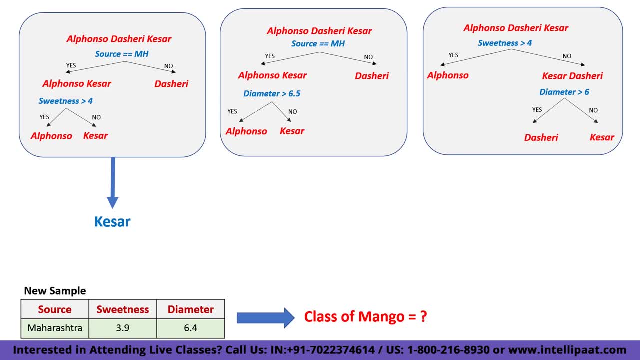 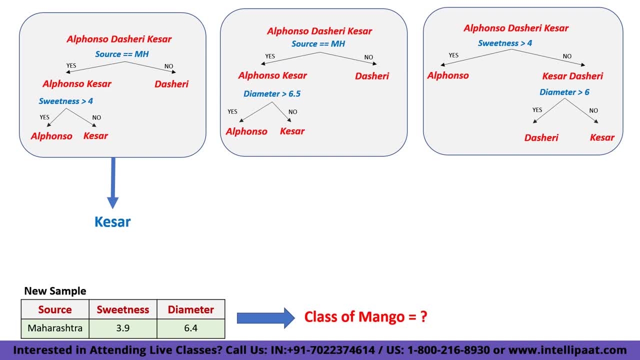 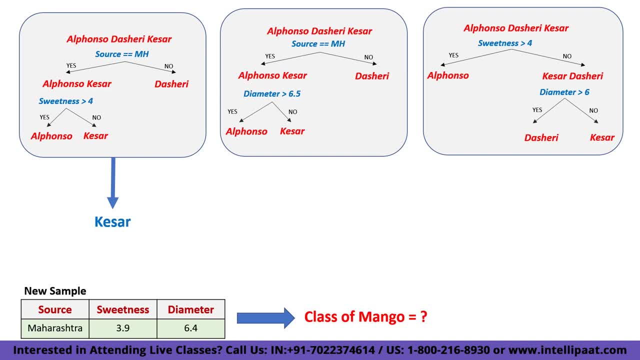 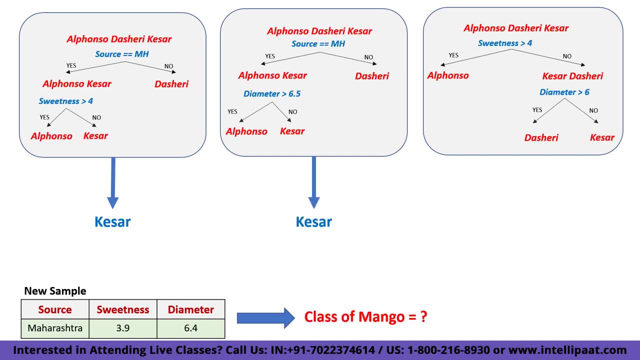 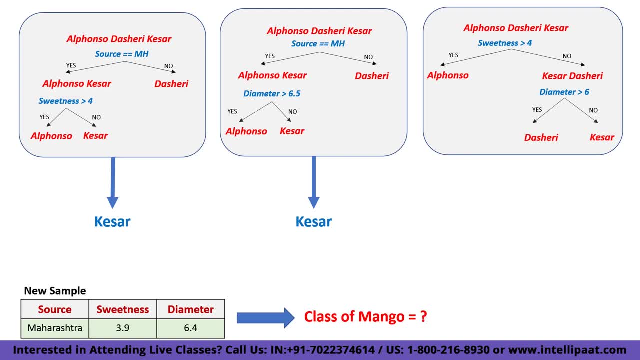 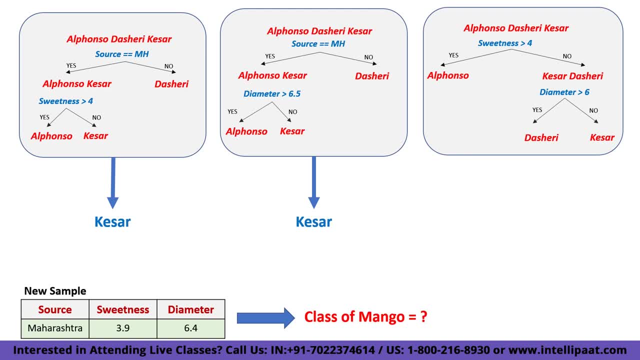 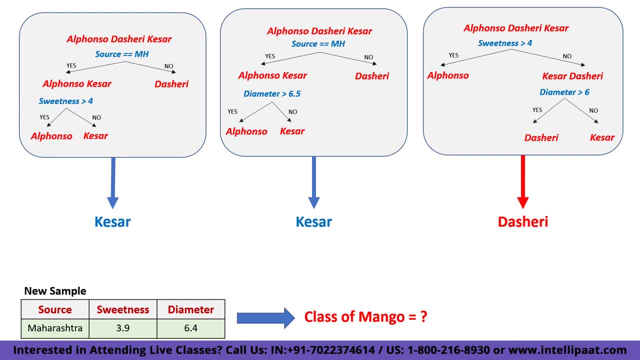 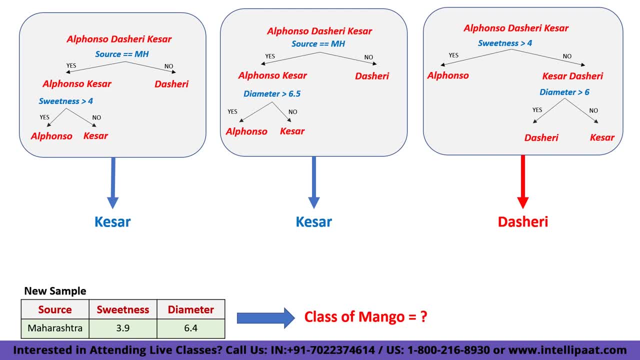 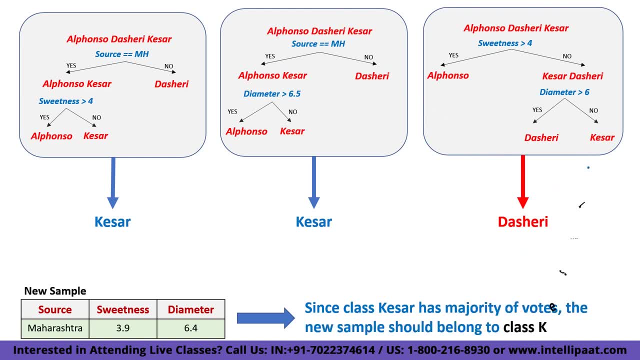 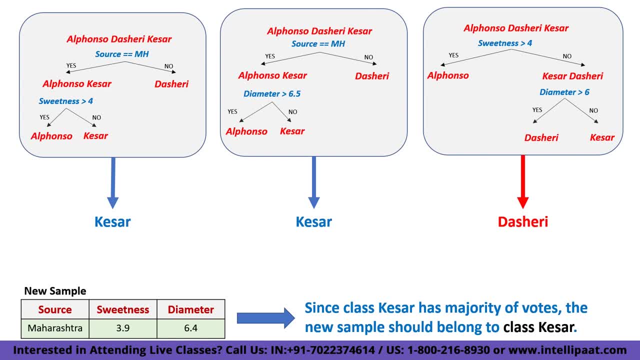 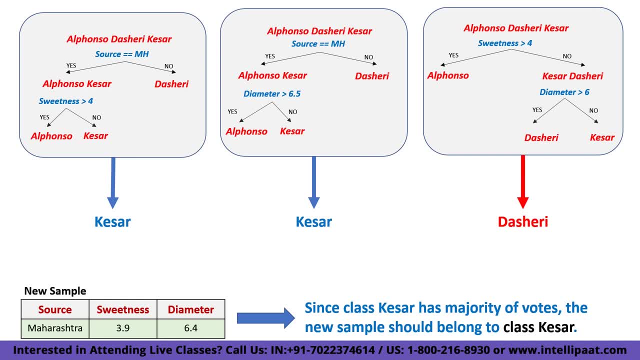 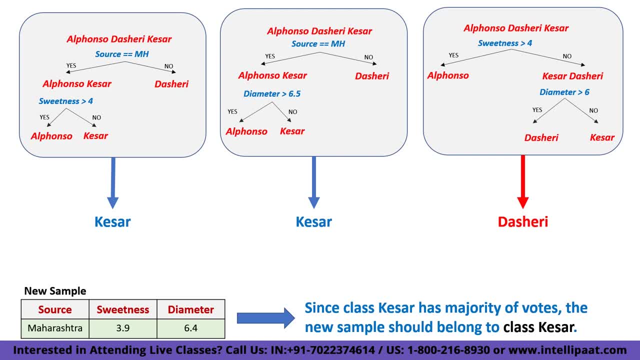 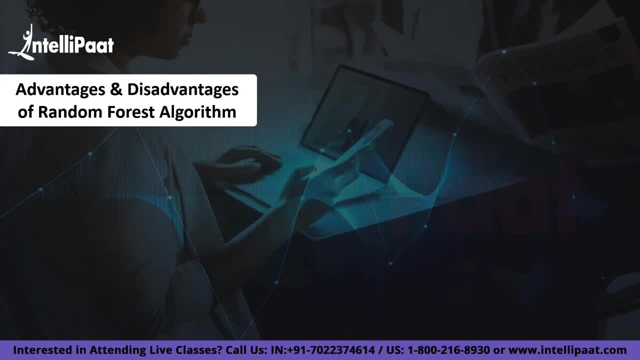 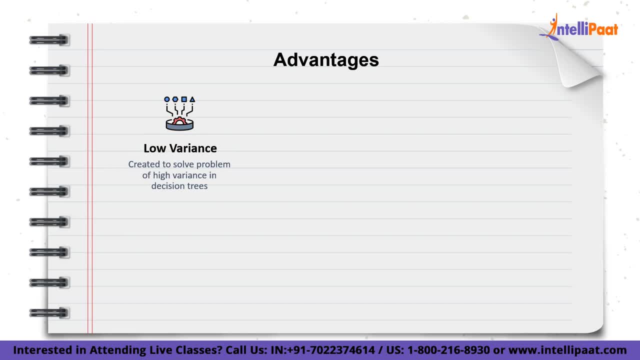 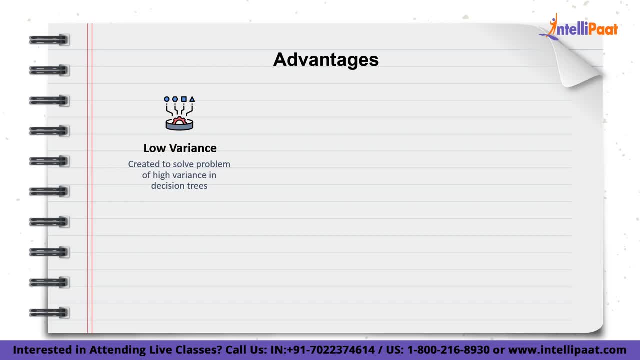 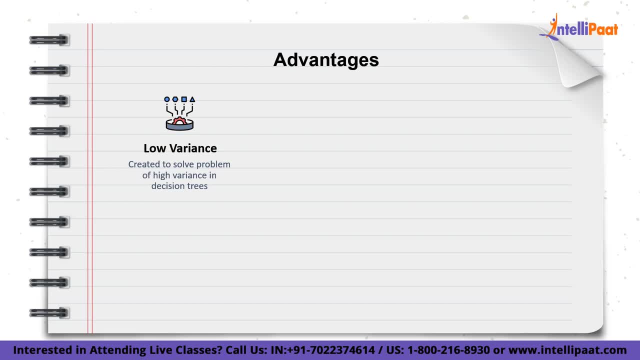 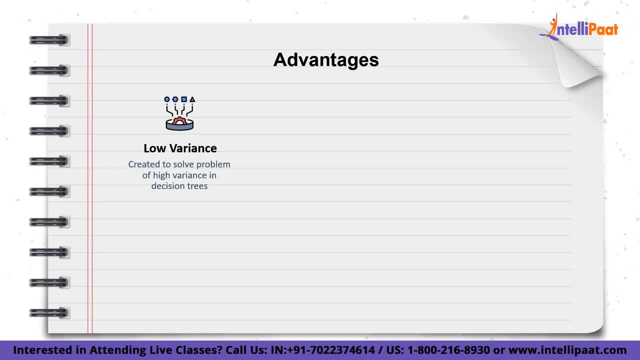 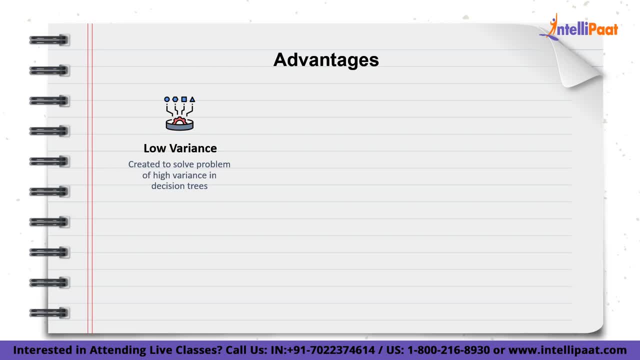 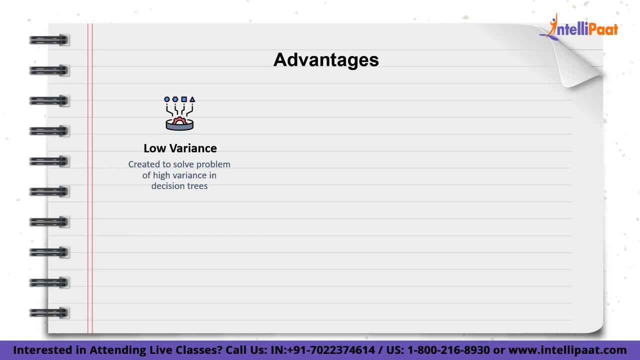 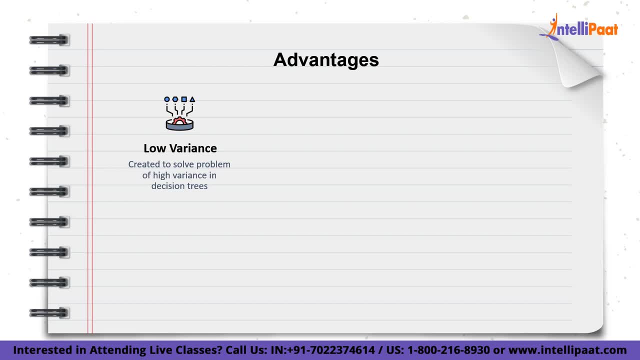 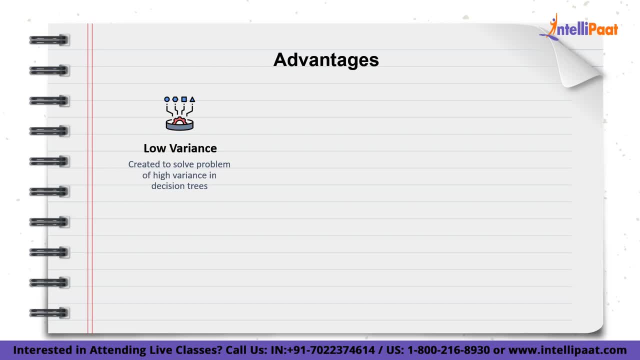 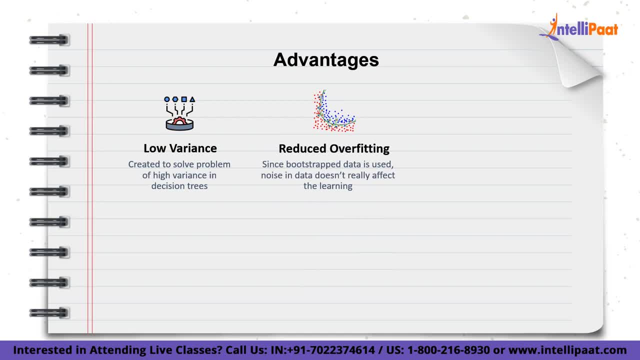 bootstrapping and aggregation. So let's start with bootstrapping and aggregation. So let's start with bootstrapping and aggregation. So let's start with. we use small bootstrap data samples to create decision trees. So definitely, there is going to. 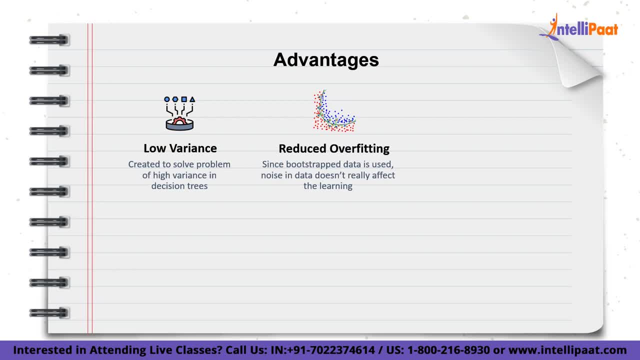 be less depth and hence very less overfitting. Also, the model won't be much affected by the noise in the data. Reason being: we generate a multitude of trees to drive the single decision right. Another advantage we have here is that, in case of this model, the normalization is not. 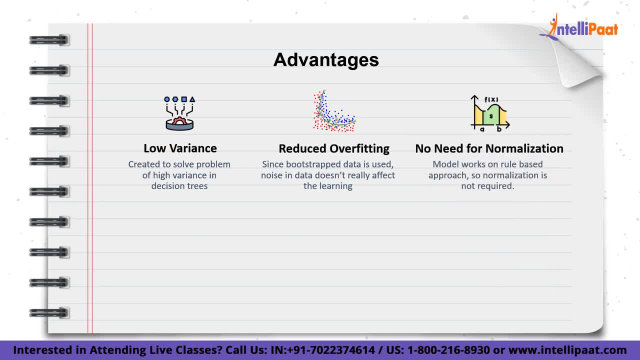 required at all. This whole algorithm works on a rule-based approach, So definitely there is no need to worry about different ranges available in the data set. Next advantage we have here is high accuracy. Random forests are known to produce highly accurate models, often outperforming other. 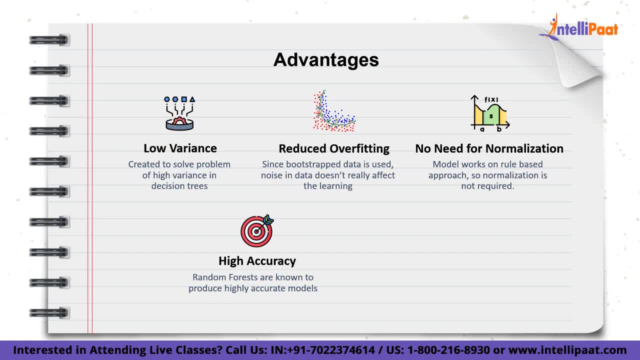 algorithms on a wide range of classification and regression tasks. Fifth advantage I have here is scalability. Random forest can be easily generated by the use of random forest. So if you have a random forest, you can easily parallelize and distribute it across multiple processors or 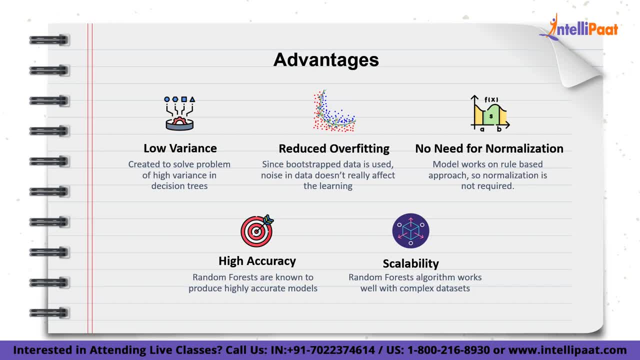 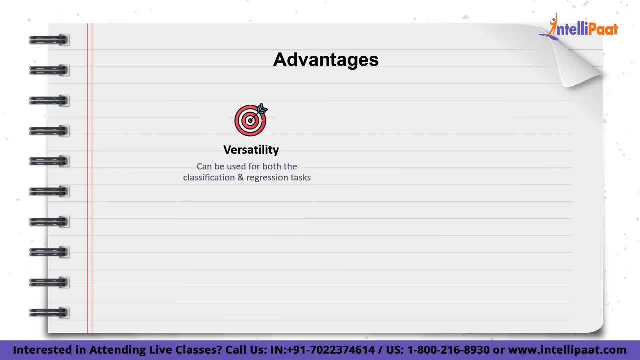 clusters, making them scalable and efficient for huge and large data sets. Next advantage we have here is that the random forest algorithm is quite versatile. This algorithm can be used for both classification and regression tasks and can be applied to wide range of problems in various industries. Hence it is considered as CART algorithm as well. 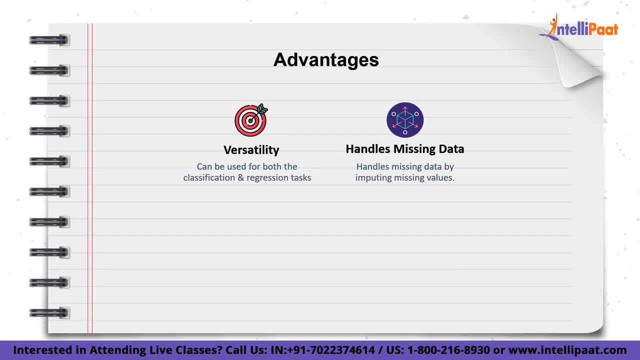 Next advantage we have is random forest can handle missing data by imputing the missing values, which can be useful for real-world data sets that often contain missing values. Okay, those were advantages of random forest algorithm. Let me also cover some of the pitfalls this algorithm brings to the table. First disadvantage I have over here is complexity. 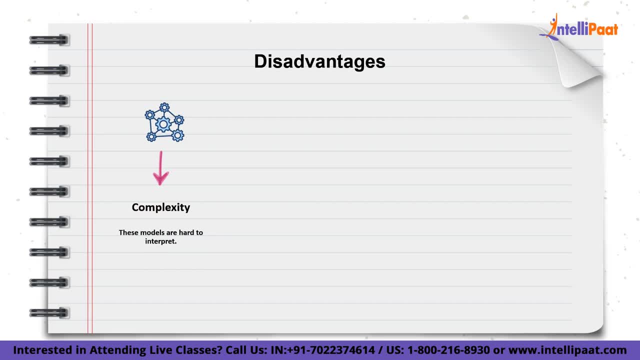 Random forest algorithm can be complex than other algorithms such as linear regression, logistic regression, decision trees. because they are built from multiple number of decision trees, This complexity can make the model harder to interpret and explain to others. Another disadvantage about random forest that we have over here is it is computationally expensive. 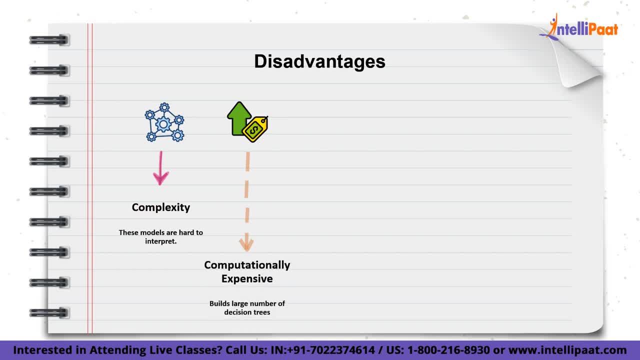 Random forest can be computationally expensive to train and evaluate, especially for large data sets with many features. Random forest can be computationally expensive to train and evaluate, especially for large data sets with many features. This is because the algorithm builds a large number of decision trees and combines their predictions, which can be very, very time consuming. 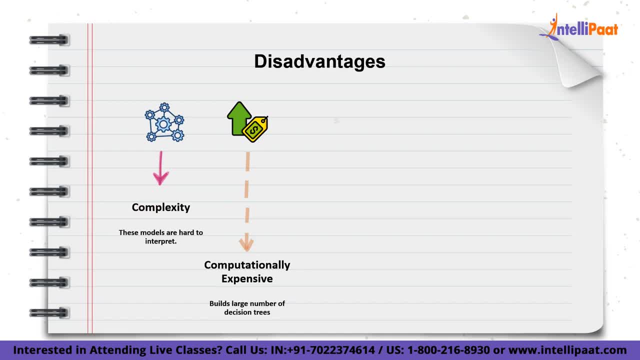 Third disadvantage that I have over here is that random forest can become biased towards features with many levels, The reason being these features tend to have more splits and therefore more opportunities to improve the model's accuracy, Sub-optimal feature selection and poor generalization performance. 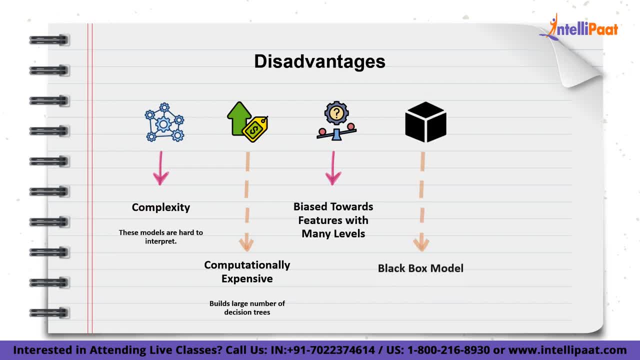 Yet another disadvantage we have over here is that random forest can be considered as a black- box model, meaning that it can be difficult to study how the model arrived at it's prediction. This can make it challenging to interpret and explain the model's behaviors to stakeholders or to anyone else who wants to learn about the model. 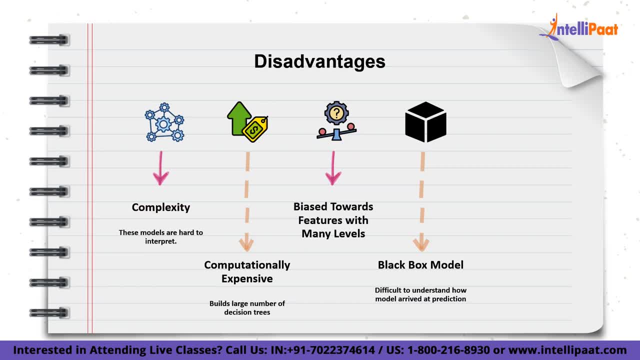 finding it to tteokbokki is. random forest cannot work better with imbalanced datasets. Random forest can struggle with imbalanced datasets where one class or outcome is significantly more prevalent than the others. This is because the algorithm can prioritize the majority class and ignore the 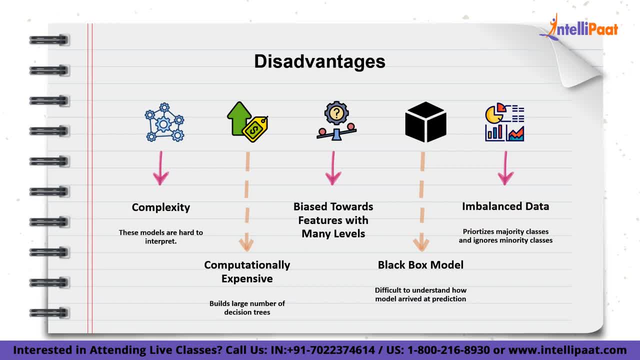 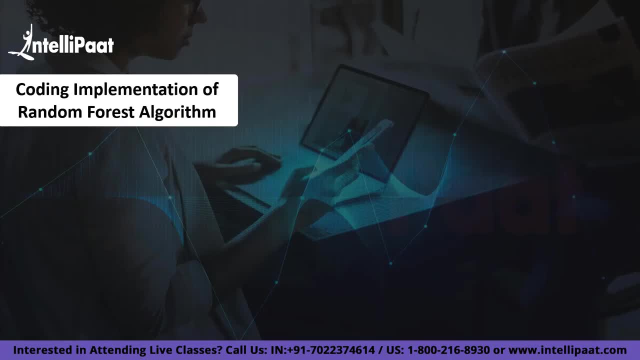 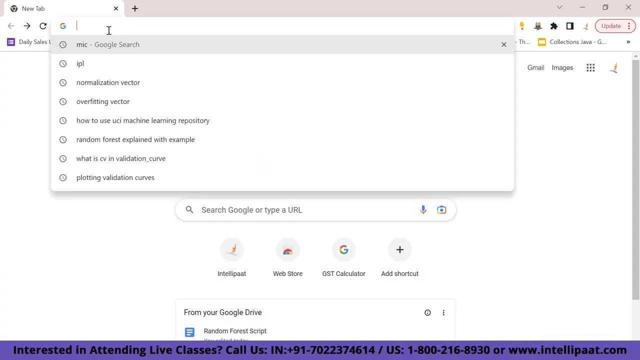 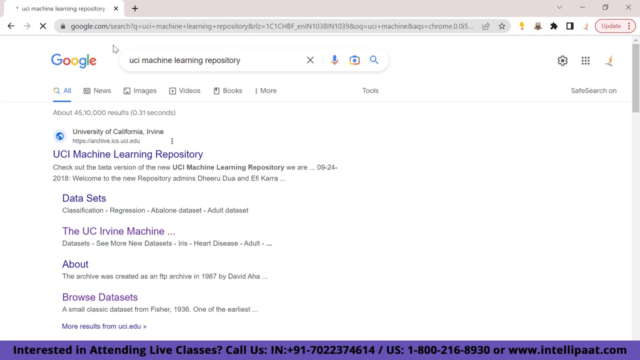 minority class, leading to biased predictions. Alright, that's all we have for advantages and disadvantages section. Moving forward, let us dive deep and construct hands-on demonstration for developing random forest algorithm from scratch. The dataset that we are going to use is available over the UCI machine learning repository, So let me first load this repository. 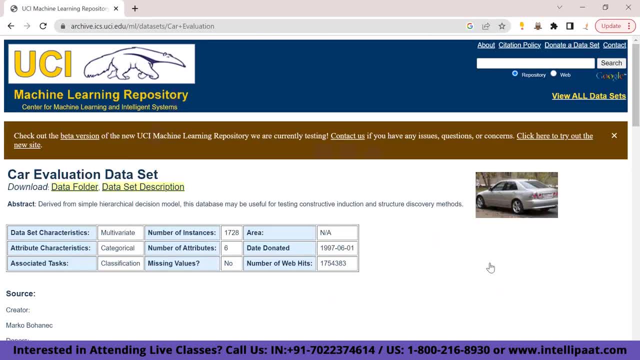 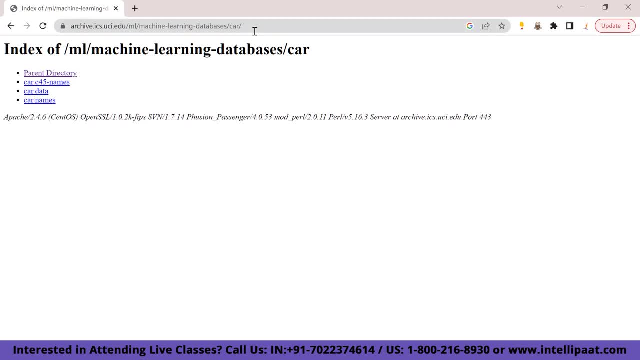 Over here. this dataset, named as car evaluation, is what we are going to use for this particular session. So go into the data folder Then copy this link, Open the Collab notebook and load the data over here. But for that purpose. 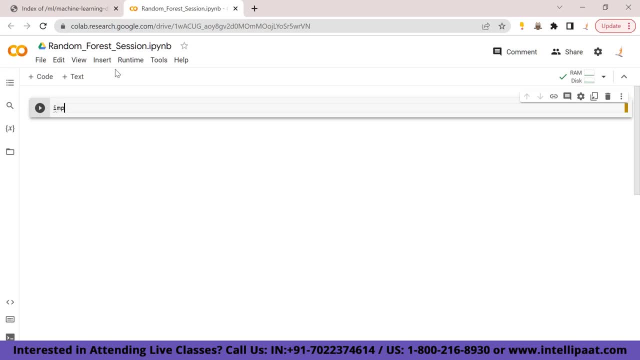 we are going to require the Pandas library. So first of all, let us import Pandas framework And then we'll save our data inside data frame and we'll use the function named as pdread underscore csv For that. we will paste this copied link into our pd library. 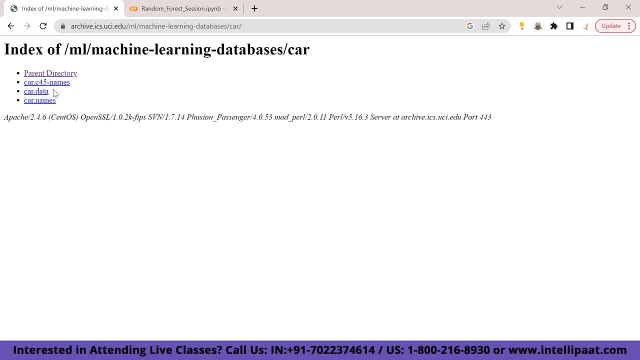 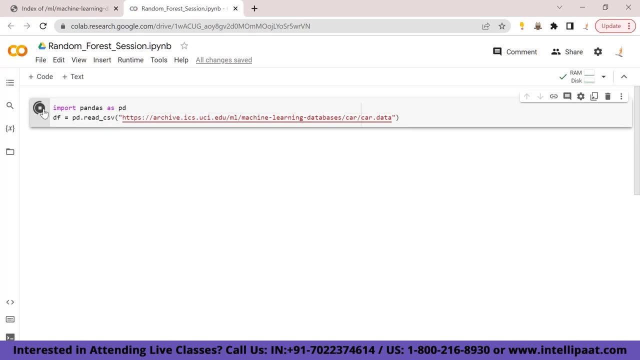 Also, we'll need the name of data file, that is, car dot data. So just copy this name and paste it over here And run this block of code And to validate if data has been loaded into your data frame or not. 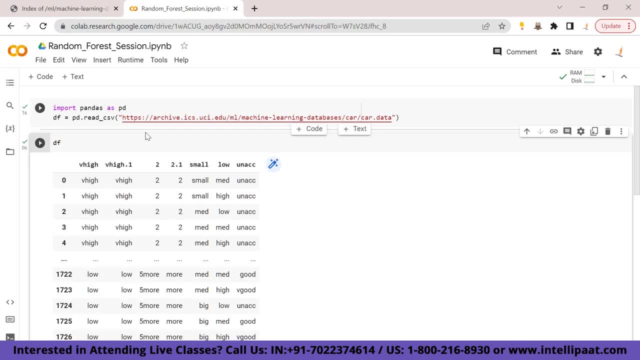 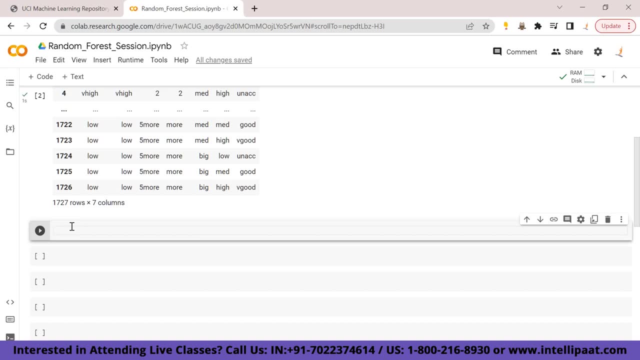 just run this block by writing tf and you will get the data over here Now. next we shall import few more dependencies that we might need down the line. First I'll import numpy framework, then I'll import seaborn. I'll also import the matplotlib framework and I'll run this block Now. next, I want you. 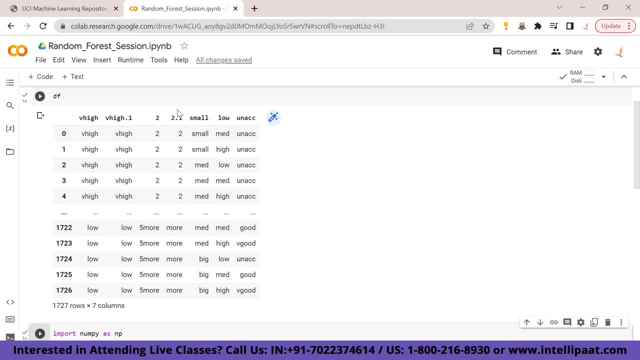 guys to notice that we really don't have proper column names for our data set. I mean, you can clearly see that data starts directly with the first row, so we definitely have to do something about it In order to comprehend this data set. Alright, let us visit UCI directory to know more about. 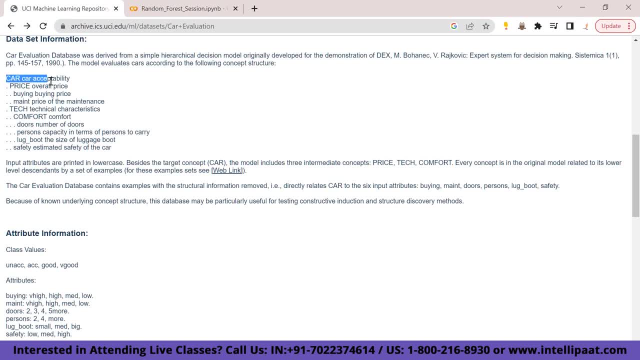 the data set Here, we can see that this data basically highlights whether the car is acceptable or not. The target variable for this data is going to be class, which highlights the acceptability of car. The values for this target variable are unacceptable- acceptable. 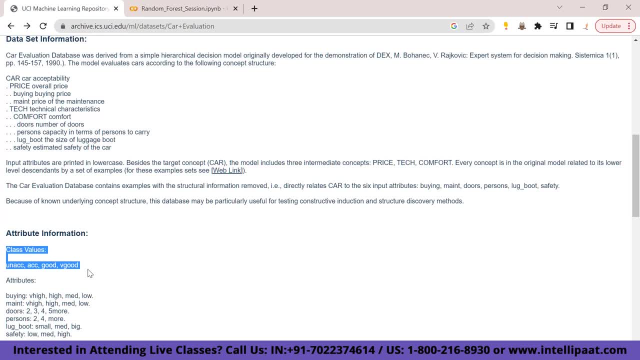 good and very good. Besides that, we also have six different features named as buying, mint, doers, persons, luxury, boot and safety. The buying attribute over here represents the buying price. Next, the doer attribute represents the number of doers the vehicle has. Similarly, the persons attribute represents 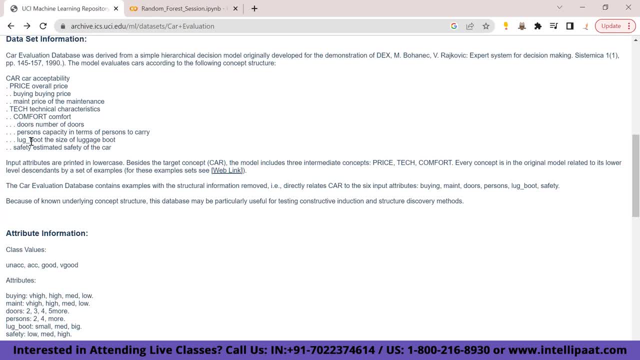 the number of persons vehicle can carry. After that, we have lug boot, which is the short form for luggage boot, and this represents the size of luggage boot that the particular vehicle have. And the final attribute, safety, provides categorical information about safety of car. Alright, so now we know the different columns available in our data set and what actually 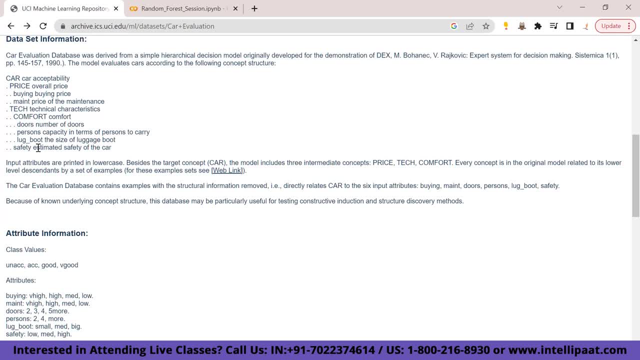 we want to do with this data set. This is simple classification problem where we'll have to classify. We'll have to classify the given car samples into the four categories that we mentioned earlier. Those categories are unacceptable, acceptable, good and very good, So moving. 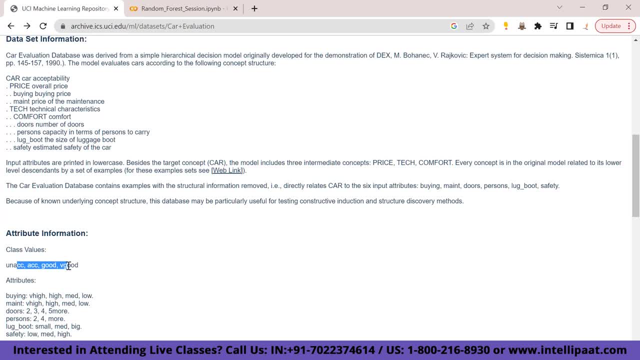 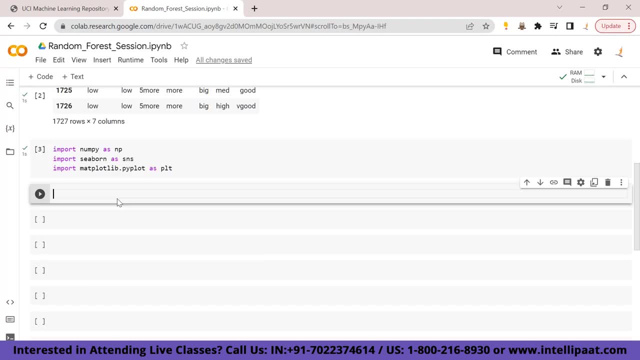 forward. let's visit our colab notebook and provide perfect titles, that is, column names, to our data set For that purpose. what I'll do here is I'll create the list of titles and I'll name this as column underscore names And inside it. 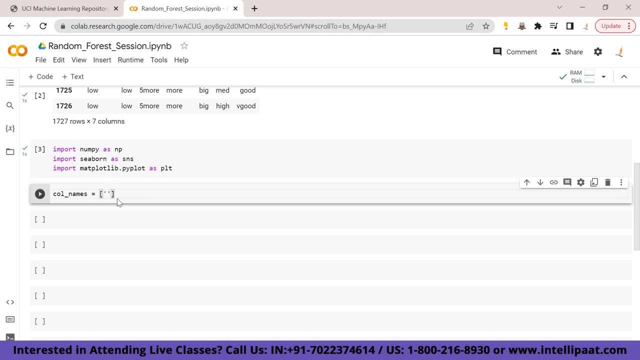 I'll put column underscore names. I'll put all the titles one by one. The title for first column was buying, Then we had mint, Then doers, Then persons, Then lug underscore boot, Then safety And then the last one. 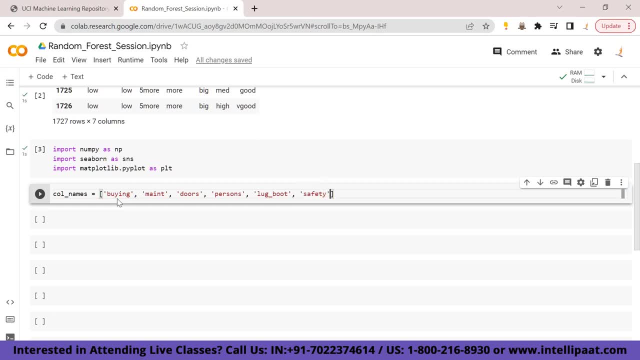 And then the last one, And then the last one, And then we had target variable, that is class. All right, Now what I'll do is I'll simply use the dot columns attribute of data frame and we'll set it equal to column underscore names list. 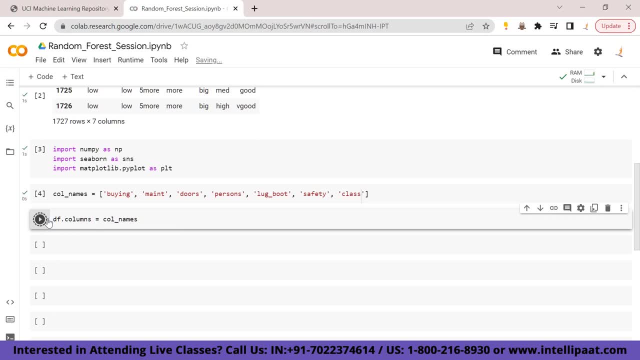 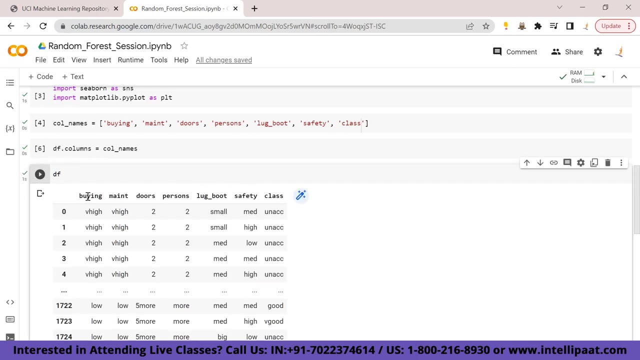 And this shall change the titles of all the columns in our data frame. And to validate that, what we'll do is we'll print our data frame And here you can see that all the column names has been applied to our data set. All right, 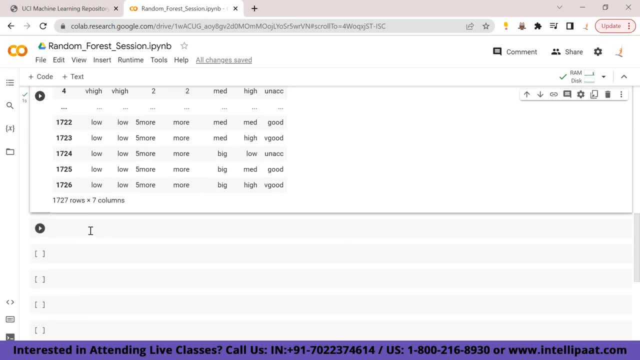 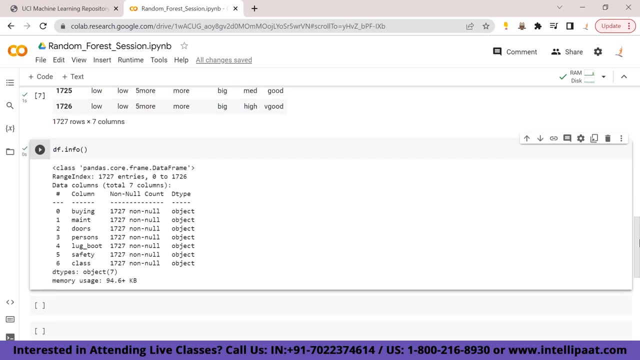 Now let us learn more about our data. First, Let us put info function to use over here. With these info function, we'll get to see if there are any null records available inside our data or not. And here we can see that there are overall 1727 entries in our data set. 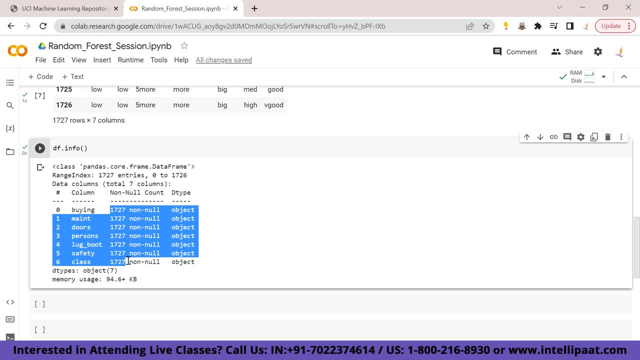 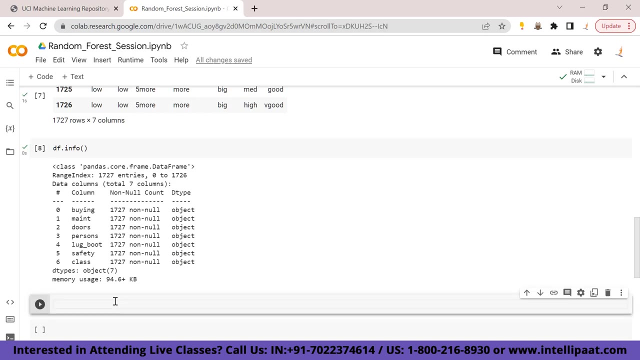 And we have 1727 records for each column. So what that represents is we don't really have null objects available inside our data. also, the data type for all of our columns is of object type. Alright, now moving forward, let us know about total number of unique values across each. 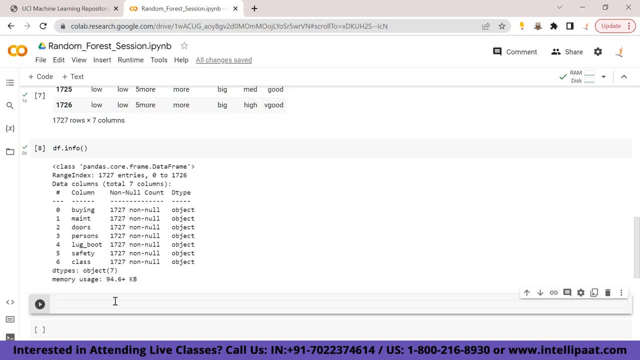 column, along with details such as the most frequently seen records and their frequency. In order to get this done, we'll use dfdescribe function over here and inside it. what we'll do is we'll set include parameter to all, so that we'll get details about all the columns of our data set. Now, once I run. 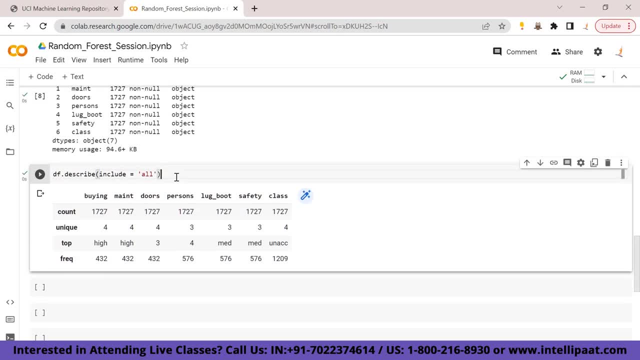 this command, but if I want them to be represented in a well-managed tabular format, then what I'll do is I'll just take a transpose of this and see the records. this way seem like much subtle, Aren't they? And here you can observe that we have 1727 records for each column. 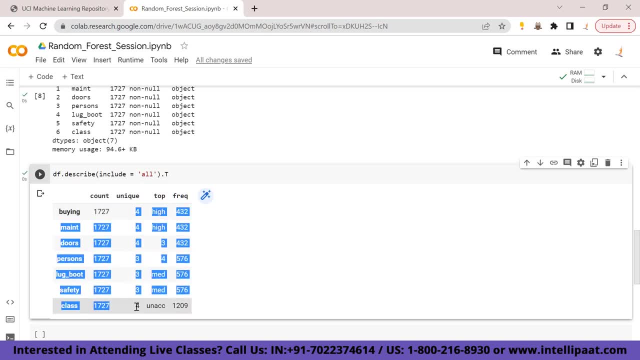 and there are different unique values available inside them For buying. we have four unique values, out of which high is highly seen inside this column. Alright now, next thing we shall do here is we shall visualize the frequencies of all unique attributes across each and every column, and it's pretty easy to do All we 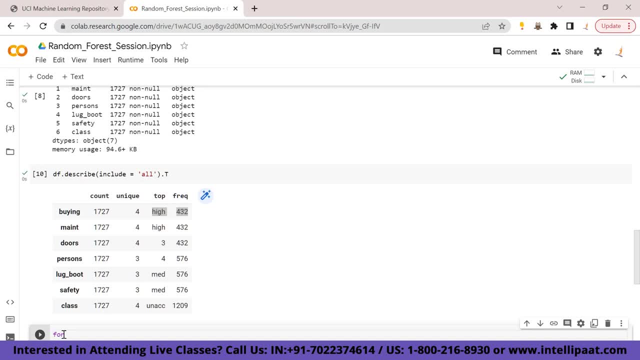 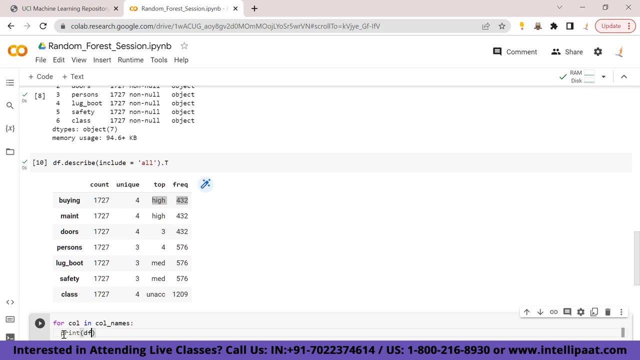 have to do here is we shall visualize the frequencies of all unique attributes across each and every column, and it's pretty easy to do. All we have to do is create a looping condition, so I'll use for loop over here and I'll just simply print the value counts for each available column. Now, once I run, 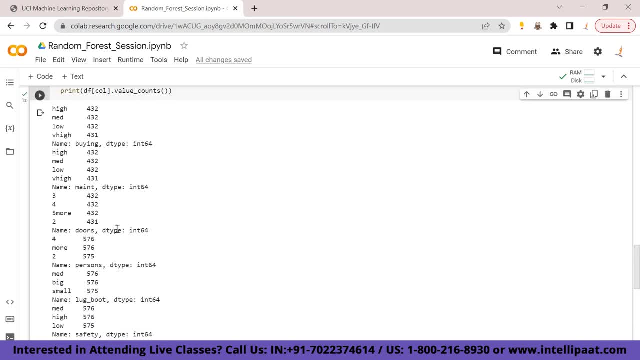 this. I'll get records about each and every individual attribute inside a column, all right. for example, in this buying column we have high, medium, low and very high as an attributes, or let's say entries, and high attribute has 432 as frequency. similarly, medium has 432 frequency. 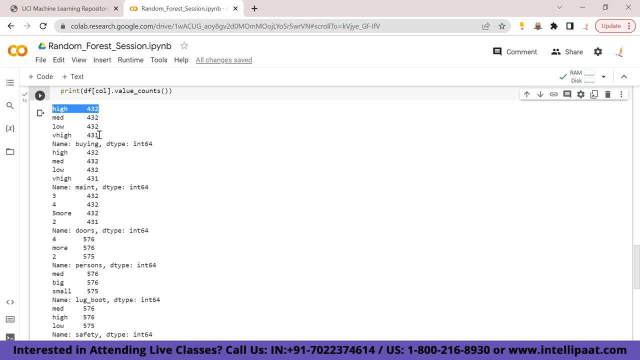 low has 432 frequency and very high has 431 frequency. now, similarly, we can see that we have got frequencies for all the samples and all the columns over here. okay, now moving ahead, what we shall do is we shall check whether, if our data contains duplicate values or not. 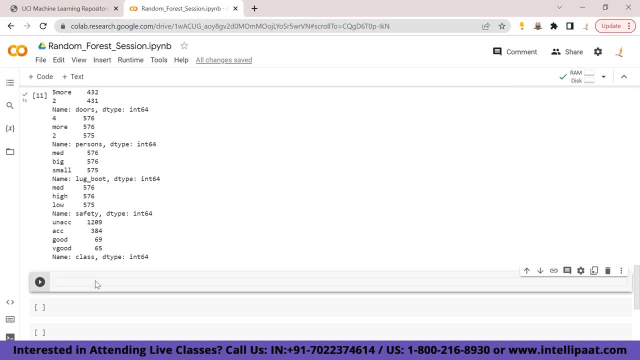 we have already checked that we don't really have null values inside our data set, so there is no need to imply is null method over here. instead of that, we'll check whether we have just check for duplicated records and for that purpose we have function named as duplicated. 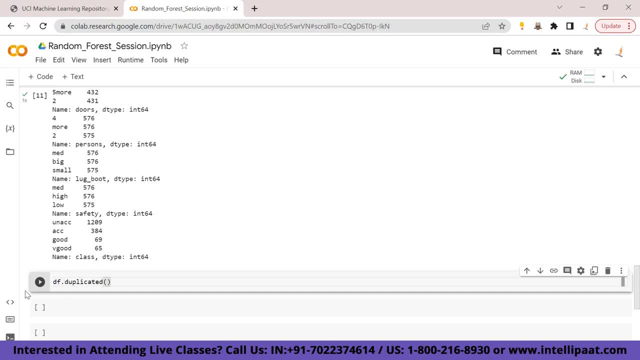 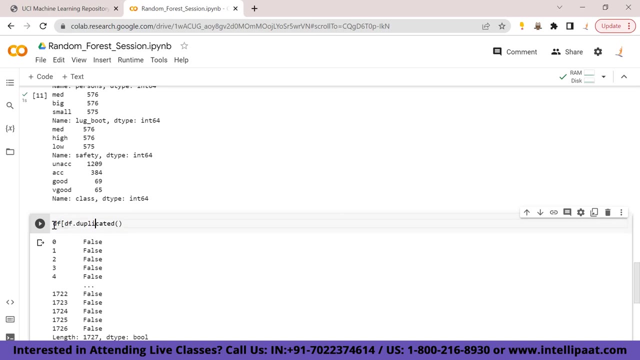 so this function over here returns the true, false, that is, boolean series object for whole of our data set. now if we just put this inside the data frame, then we shall get only the records which are duplicated on our screen. but since are getting nothing over here, we can conclude that our data doesn't really have any duplicated. 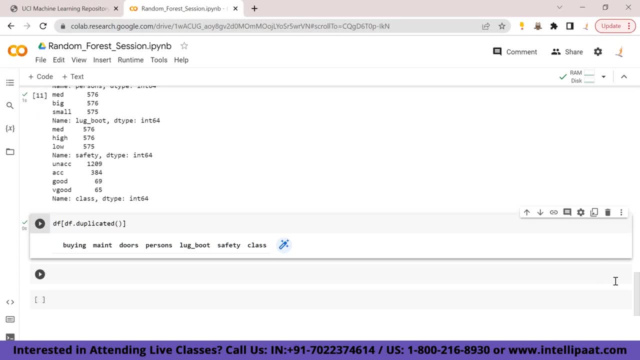 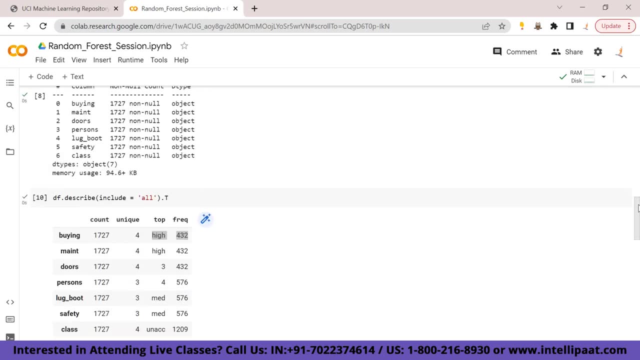 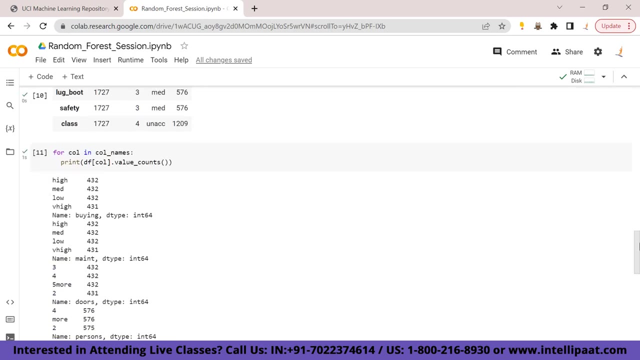 values inside it. So now the only thing that the left over here in pre processing phase is dealing with non numeric values. we saw that all of our data columns are made up of object type, So we'll have to convert them into numeric type so that we'll be able to feed them to the 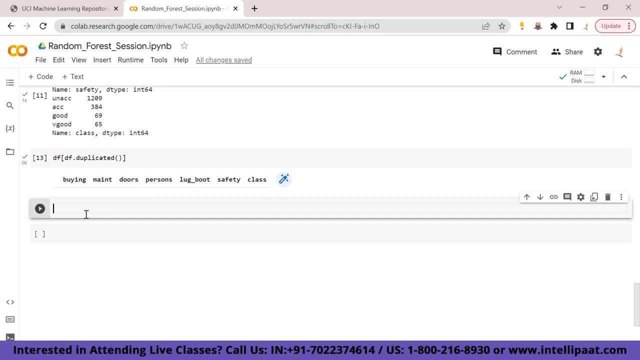 model. And in order to do that, what we are going to do is we are going to use encoding technique, known as ordinal encoder. What this encoder does is it converts the categorical values into ordinal values by assigning unique values to each attribute in a column. Okay, let us first 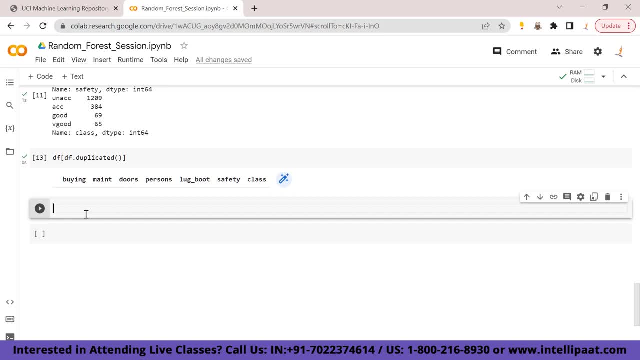 import the ordinal encoder from a skill and package to get started. So from a skill on dot pre processing, Import ordinal encoder. Now we'll create the instance of ordinal encoder. Now let us first transform the buying column inside our data frame And for that purpose, 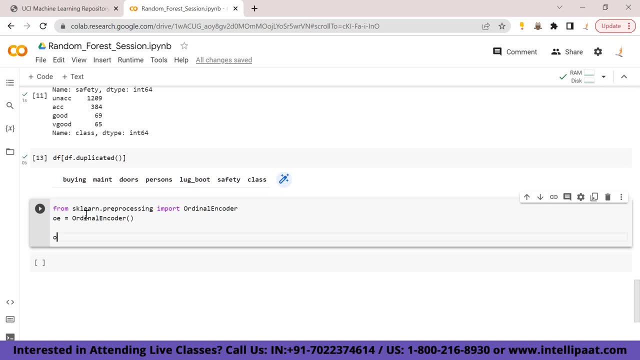 we'll use fit underscore transform method And inside it we'll simply pass the data frame as a 2d object And we'll save changes to our data frame column named as buying. Now I'll copy this line And I'll paste it down over here, because we'll just change the column names one by one. 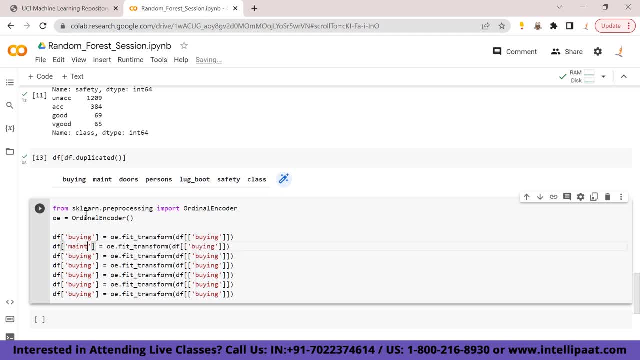 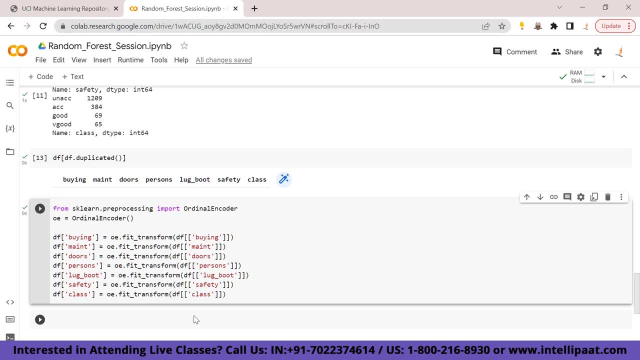 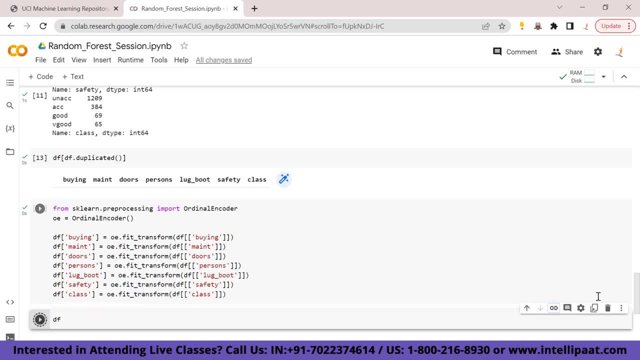 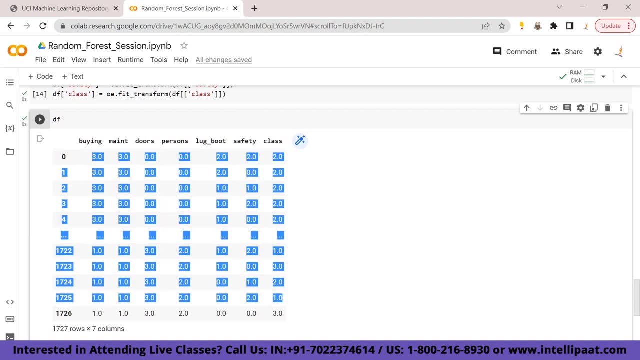 For that purpose we'll simply print our data frame over here, And here you can see that we are getting numeric records for all the columns. That means ordinal encoder has done its job. With that, we have successfully finished the pre-processing stage. 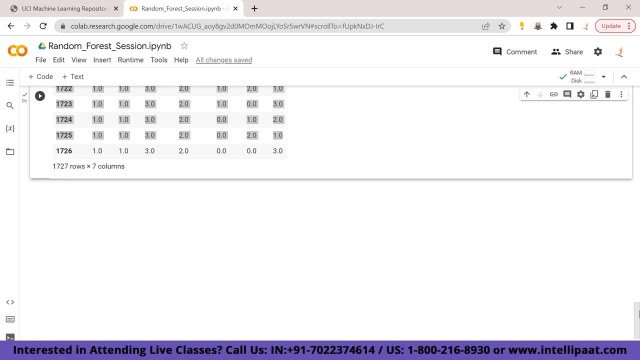 Next we'll split our data, But in order to do that first we'll have to convert it into input and output format. I'll use ilock indexing for that purpose, So I'll create input output split for first using ilock. 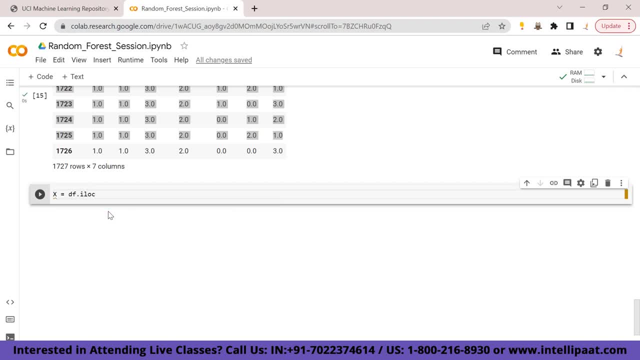 So x is equal to df dot ilock And I'll just not take the last column in our data frame And for y I'll set df dot ilock as the last column. Now we have successfully split our data into input and output vectors. 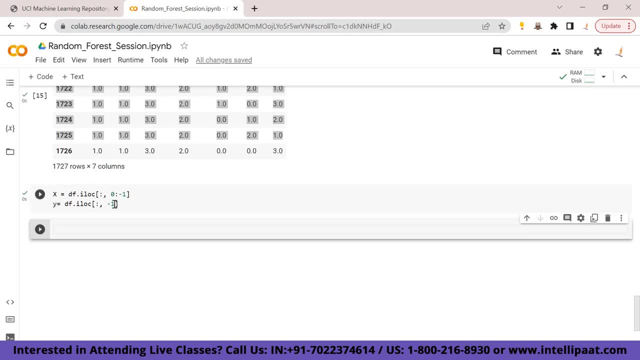 Now next thing we'll do is we'll split it into training and testing samples And for that purpose I'll import the train underscore test And this is an example of a test underscore split function available inside sklearnmodel selection package. So from sklearn dot model underscore selection. 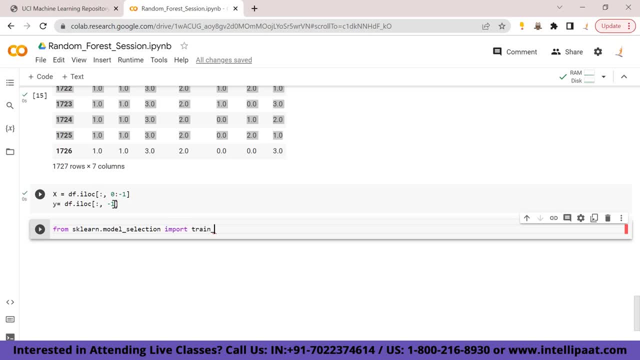 import train underscore test, underscore split. We'll set x underscore train comma x underscore test, comma y underscore test, underscore train comma y underscore test as equal to train underscore test, underscore split. here we will provide input vector, output vector, then the test size. let us set the test size as 30% and we'll set random state at 0. all right, 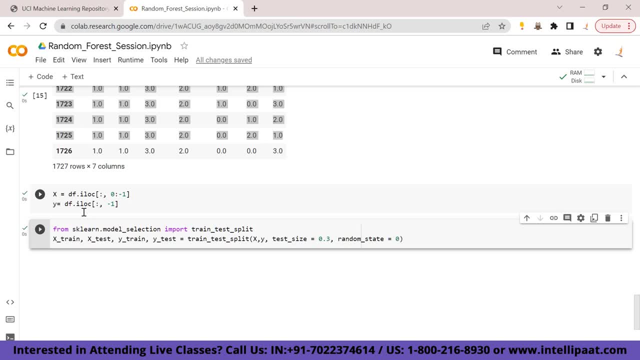 with this execution our data is ready and we can feed it to the model. so, without wasting any time, let us load the random forest classifier from a skill on dot in symbol package so that random forest classifier over here from a skill on dot ensemble import random forest classifier. now I'll create the instance of random forest classifier. 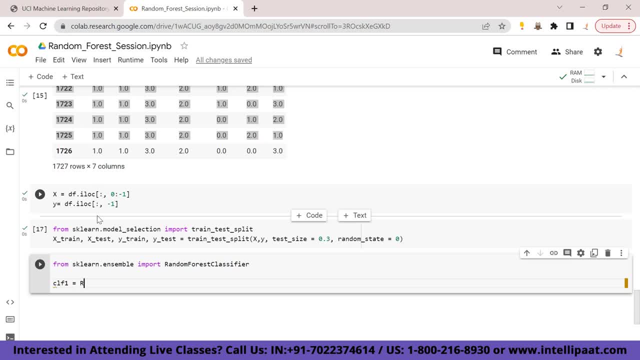 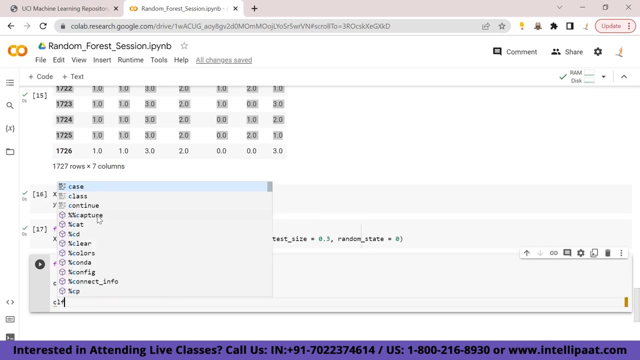 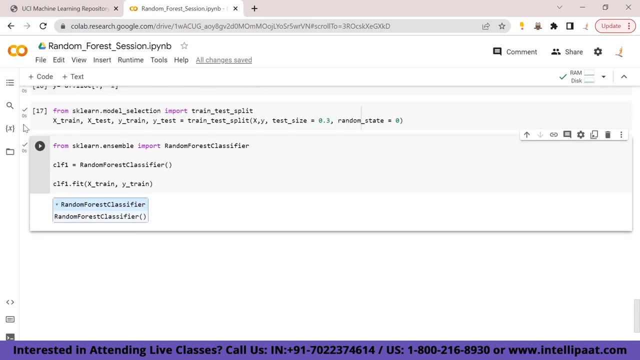 over here and basically fit my data to this classifier, Clf1. dot. fit X underscore train, comma y underscore train. now let us make prediction using the dot predict method. ok, So clf1.predict x underscore test and we'll save it inside the variable named as spread1. 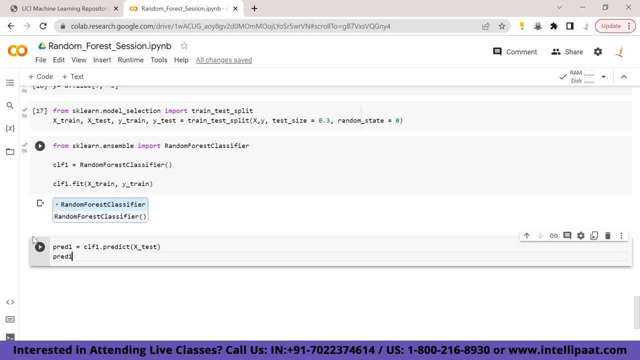 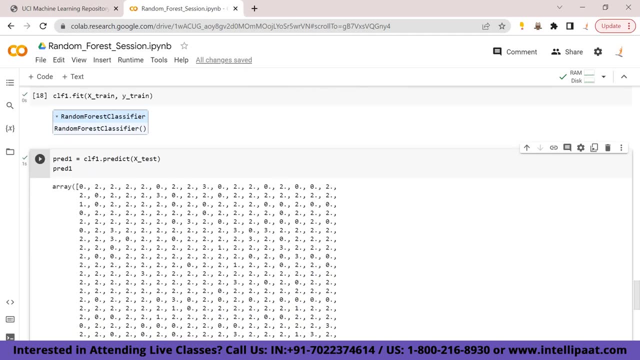 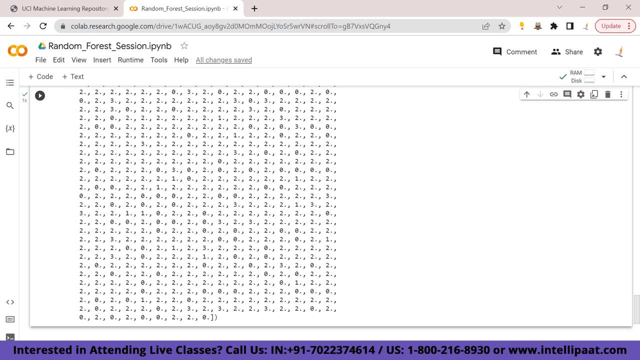 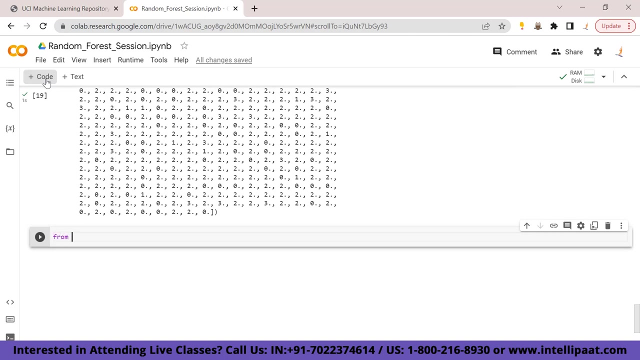 We'll also print this spread1 to see the predictions. All right, here you can see that our model has successfully predicted the results for testing sample. So let us evaluate accuracy for this particular predictions. So I'll import the accuracy score from sklearnmetrics. 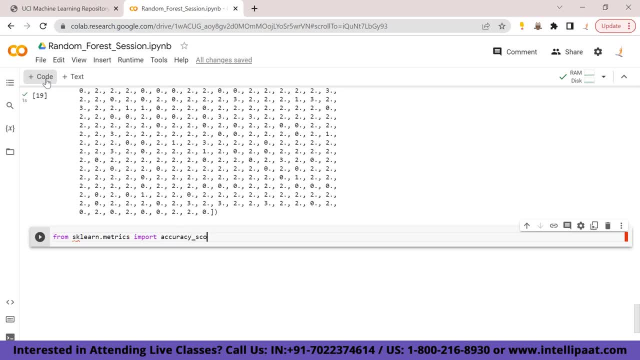 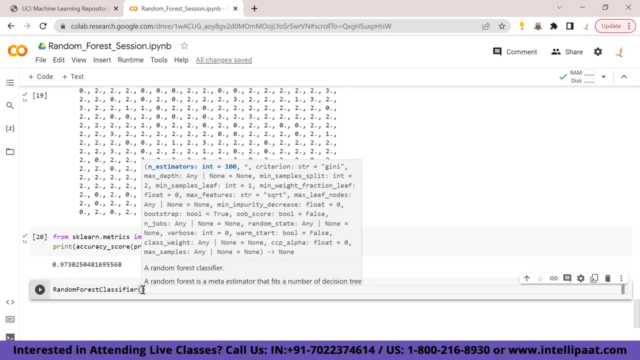 And I'll print accuracy score by comparing the spread1 and ytest. And here you can see that we are getting 97% accuracy, which is really good in the context of machine learning. But, Guys, the accuracy can further be increased using the process known as hyperparameter tuning. 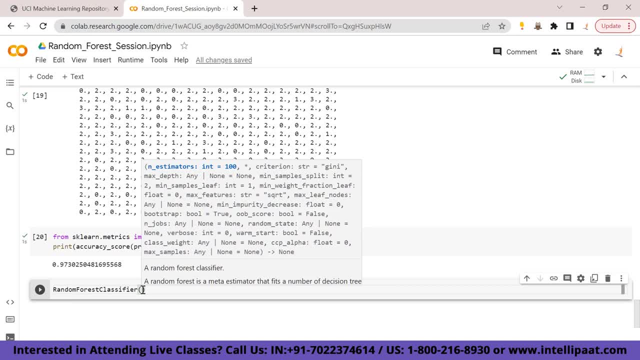 We have multiple hyperparameters in random forest, such as n underscore estimators, criteria, max depth, minimum underscore samples, underscore split, max underscore features and many more. N estimators over here represents total number of trees you want to allow inside the forest. 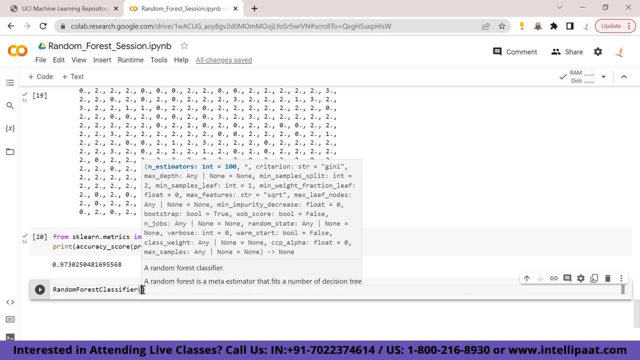 The criteria parameter over here is nothing but the methodology To measure the quality of a split. Here we have options such as gene impurity, entropy and information gain. Next parameter is max underscore depth, which determines the maximum depth of the tree. If none, then nodes are expanded until all leaves are pure or until all leaves contain less than minimum sample split samples. 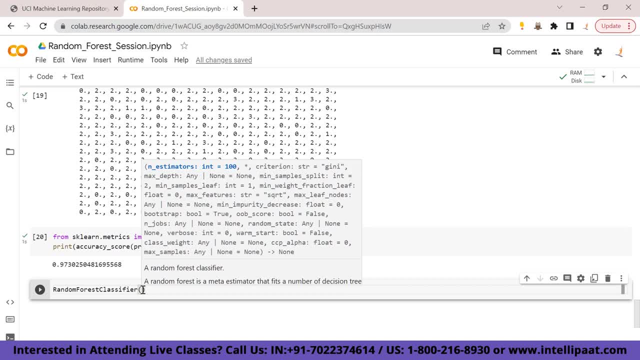 And min underscore samples. underscore split here Portrays the minimum number of samples required to split an internal node And similarly, max underscore feature is yet another parameter that represents the number of features to consider when looking for the best split. All right, But how are we going to optimize all of these hyperparameters? 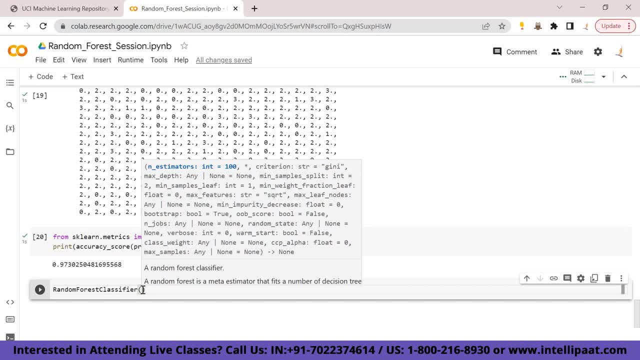 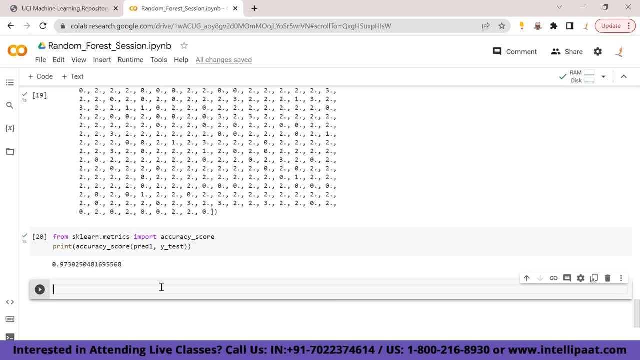 Well, there are a few methods to get optimization done. For this particular session, we'll cover the validation curve function for hyperparameter tuning. The validation curve method is a useful function in scikit-learn that helps in evaluating the performance of a model by varying one parameter while keeping all the parameters constant. 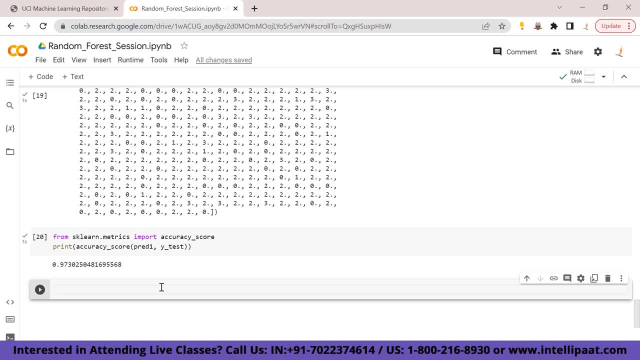 It provides insight into how the model's performance changes with different values of the specified parameter. The purpose of the validation curve method is to plot a validation curve, which is a plot of a model, evaluation scores such as accuracy, F1 score, mean, square error, et cetera, on the y-axis against different values of a hyperparameter on the x-axis. 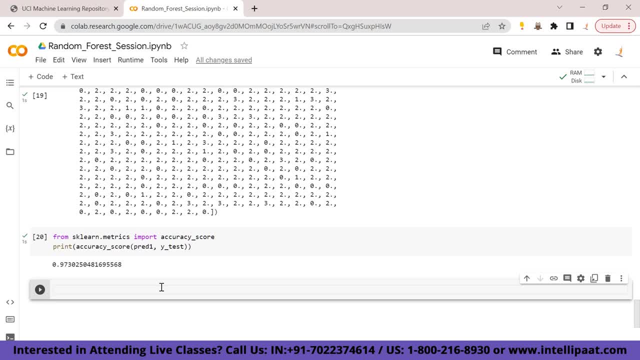 This allows us to analyze the impact of changing the hyperparameter on the model's performance and identify the optimal value. This function also contains few arguments. Those arguments are estimator x, y, param underscore, name, param underscore range, cv and scoring, et cetera. 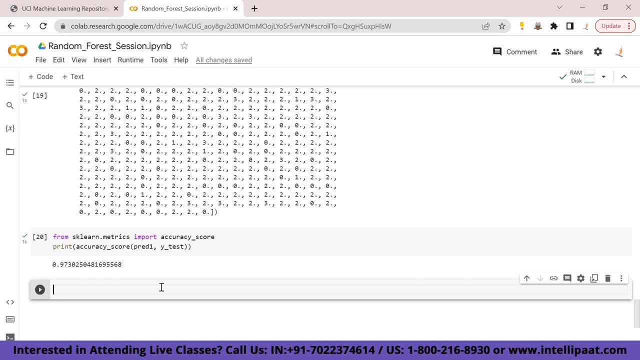 So estimator parameter specifies the model or pipeline object for which the validation curve is generated. In our case, estimator will be the random forest. X represents the input part of data. Y represents output part of the data. Param- underscore name argument is basically the one to specify the parameter of model you want to vary, while keeping others constant. 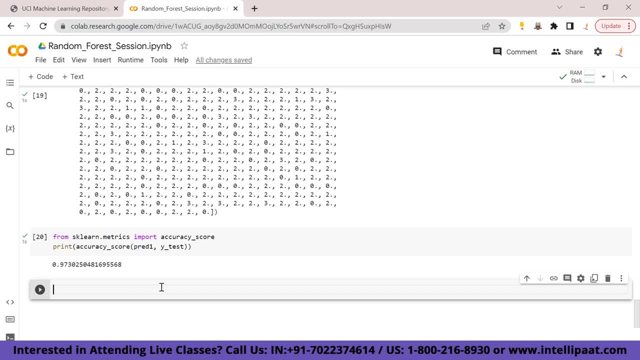 And param underscore range specifies the range. So this is the type of values for the hyperparameter to be tested. It should be sequence or array-like object that represents the different values to be evaluated for the param underscore name. Cv argument is one that determines the cross-validation strategy used to evaluate the model's performance. 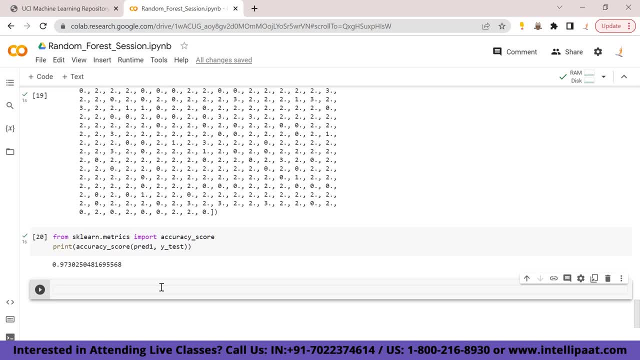 If you have three-folds, if you have five-folds or if you are using k-fold strategy. And scoring argument specifies the scoring metric used to evaluate the model's performance. And scoring argument specifies the scoring metric used to evaluate the model's performance. 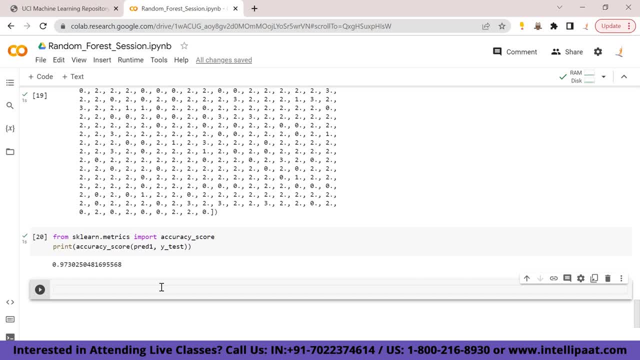 And scoring argument specifies the scoring metric used to evaluate the model's performance. It can be a string representing a built-in scoring metric from scikit-learn such as accuracy, precision, recall, F1 score, mean squared error, etc. It can be a string representing a built-in scoring metric from scikit-learn such as accuracy, precision, recall, F1 score, mean squared error, etc. 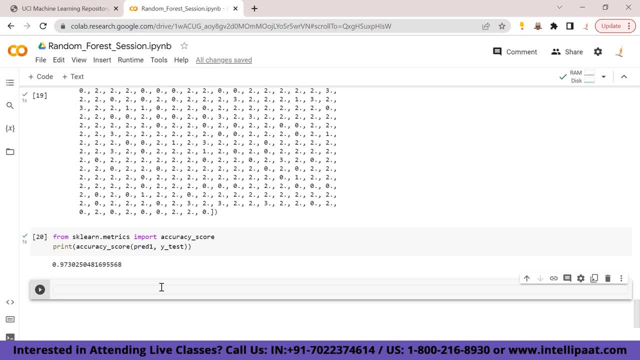 Now let me load this function and show you how it can help you visualize the accuracy for particular varying parameter. So for that purpose we are going to use visualization library named as yellow brick, And from it we are going to use package named as model underscore selection. 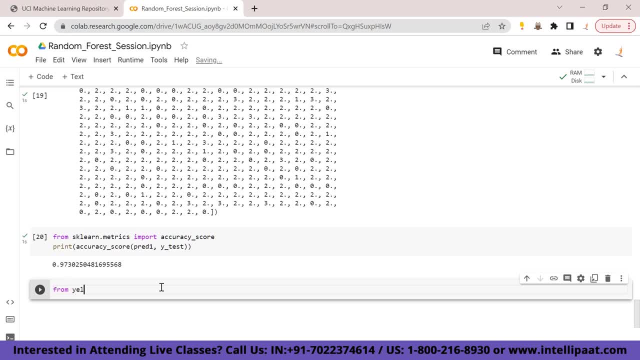 So from yellow brick dot model underscore selection import validation curve. So from yellow brick dot model underscore selection import validation curve. Now what we will do is we will create the param range. Now let us arrange this as num estimators. 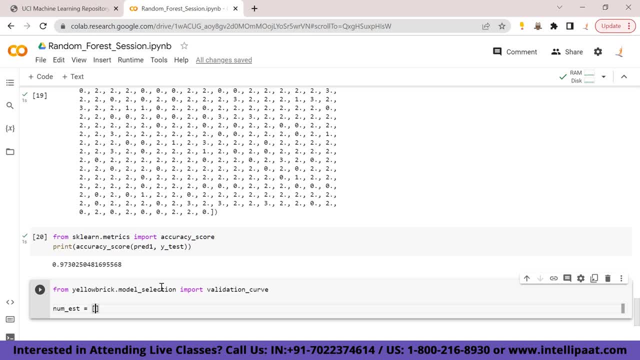 And inside it We will store random values that we want to apply to our number of trees. So basically, num estimator is going to be the number of trees we want our model to create. So initially, let us say we want to create 100, 200, 450, 500, 750 and 1000. 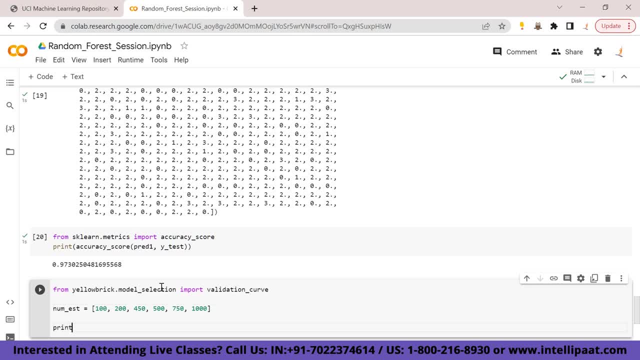 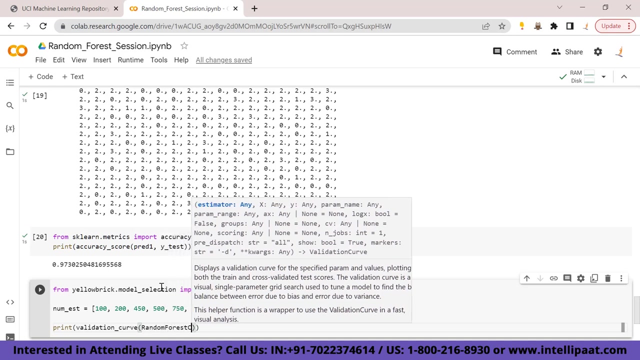 Alright, Now let us print the validation curve. So we will use validation curve function inside the print statement Because ultimately we want to return it on our console. So that's why we are using it with print function Now here. first we will provide the estimator, that is our random forest classifier. 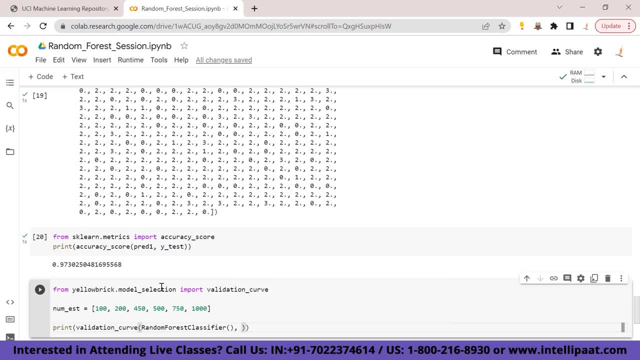 We will set x equal to x underscore train. We will set y equal to y underscore train. Param underscore name will be n underscore estimators for this particular snippet. Then we will set param range as num underscore estimators. Then scoring will be accuracy and we'll set cross validation for three folds. 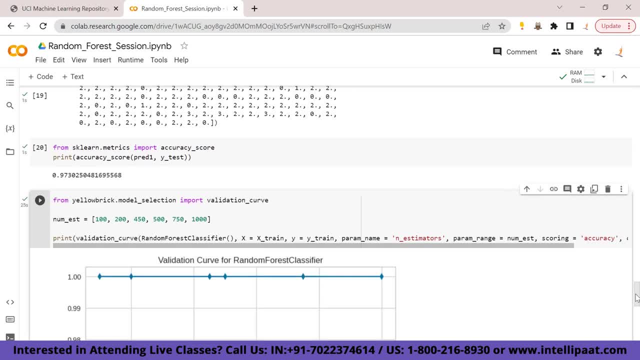 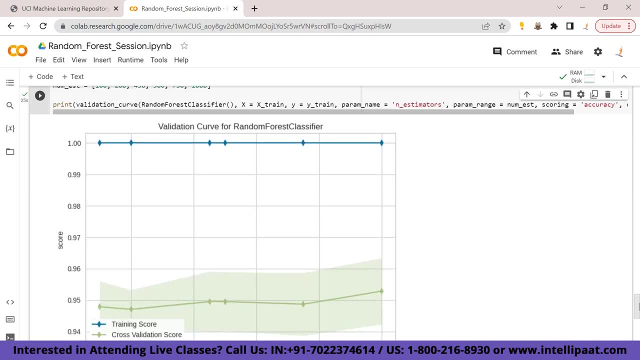 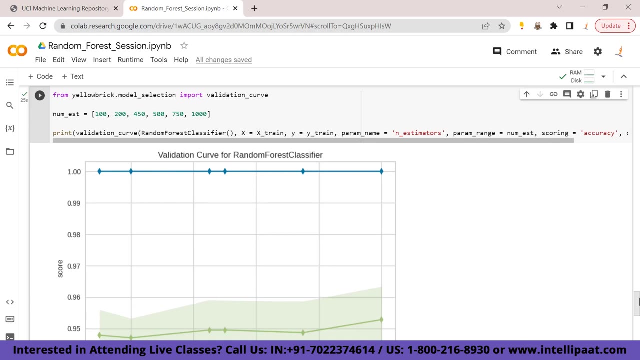 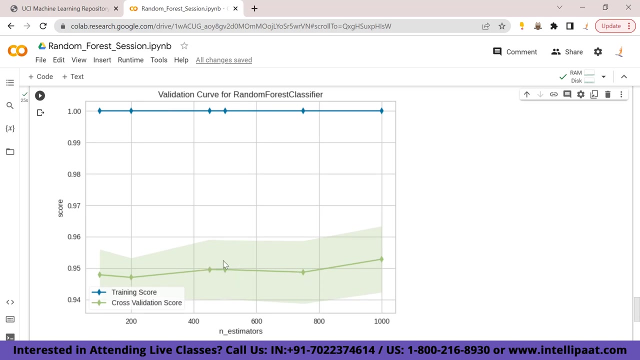 Now let us run this block of code, and here you'll get this nice graph representing how the learning is happening by keeping this parameter in mind. Now remember that all other parameters are constant, so they are not actually affecting the learning over here. So basically, in training sample, the point where we get maximum accuracy is going to. 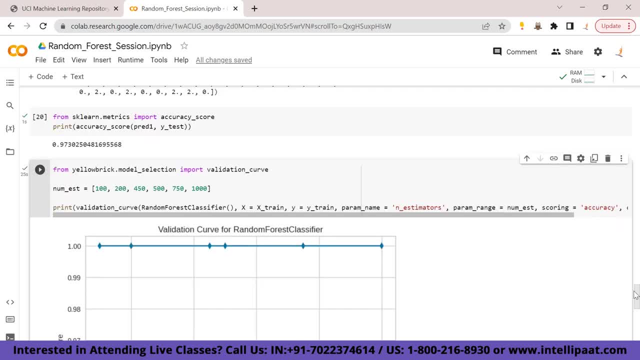 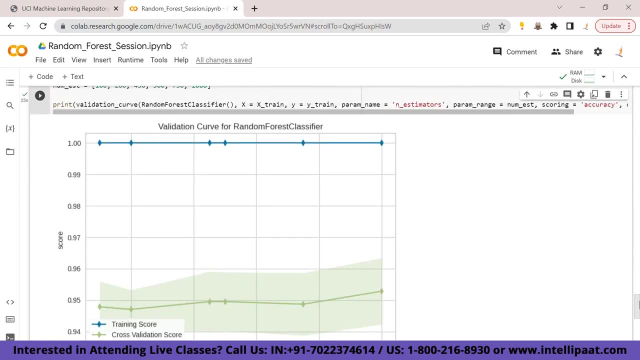 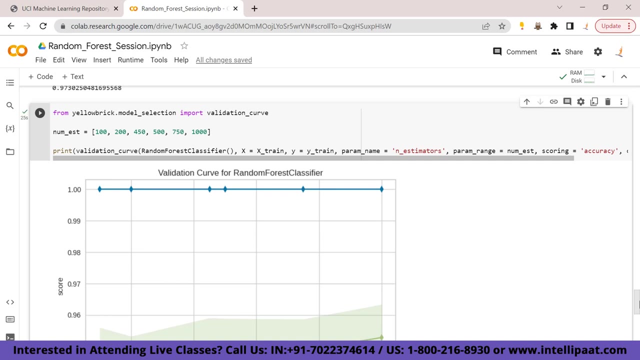 be the suboptimal value of our estimator parameter, All right. And in this graph you can see that for value thousand we are getting the maximum amount of accuracy. So what we'll do is We'll set number of estimators equal to thousand and another classifier that we'll create in 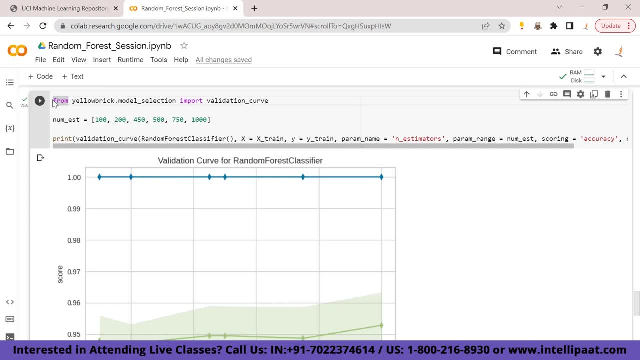 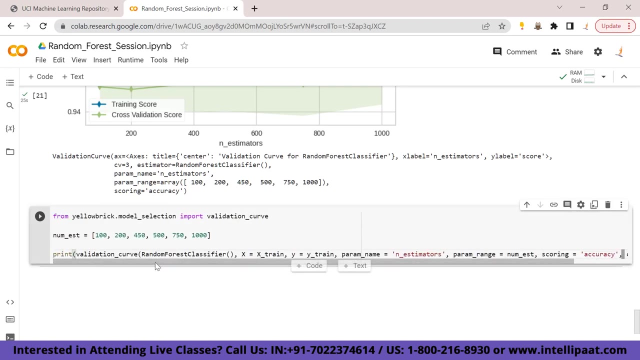 a file. But before that let us perform hyperparameter tuning for few more parameters that we have inside our random forest classifier. So I'll simply copy this code, I'll paste it here and now I'll just change the name of parameter over here. 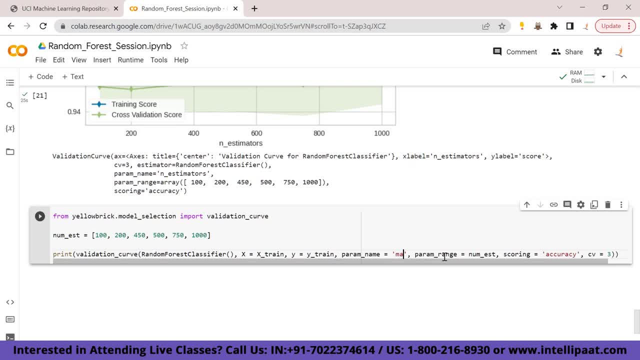 So now, Okay, We shall use max underscore depth for optimization over here. So max depth is basically going to be the height of our tree or the depth of our tree. So let us provide values such as 10,, 7,, 15,, 12,, 20 and 22.. 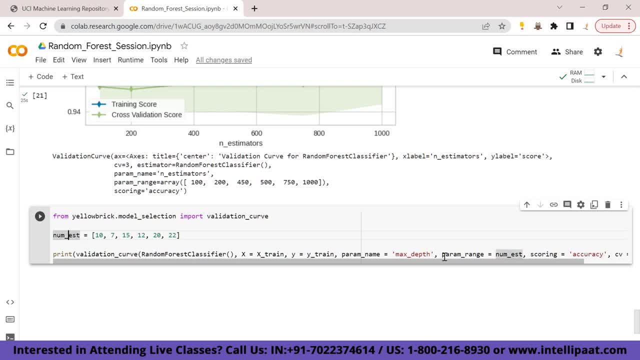 I'll change the name of this variable over here, Okay. Okay, I'll set it as depth valves and I'll update the range over here, as everything else is going to be same. So I'll run this block and here we can see that for the depth value 15, we are getting 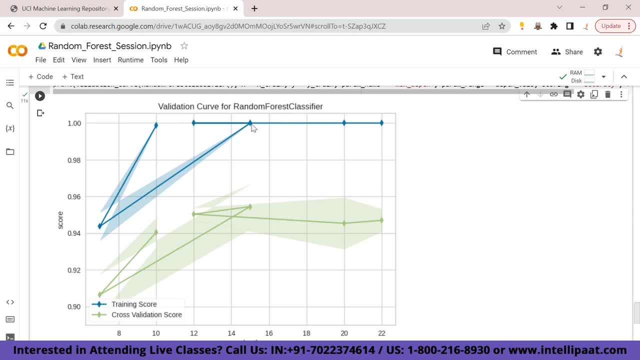 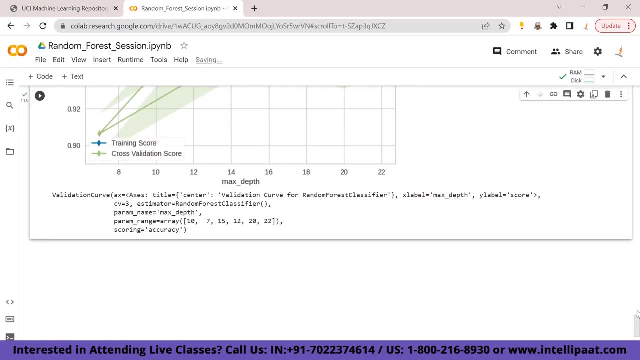 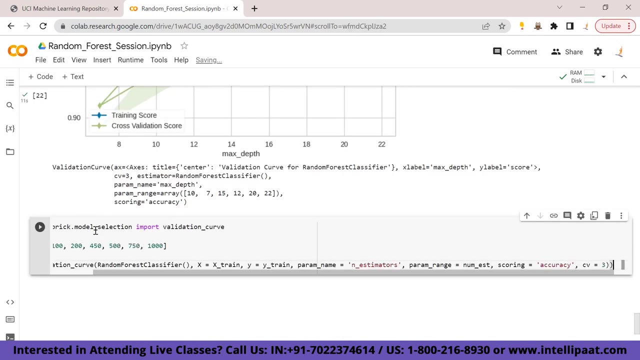 highest training accuracy as well as testing accuracy. So, definitely, the 15 is going to be the optimal value. Okay, So this is the optimal value for max depth parameter. All right, Now let us do the same for yet another parameter named as minimum underscore: samples underscore. 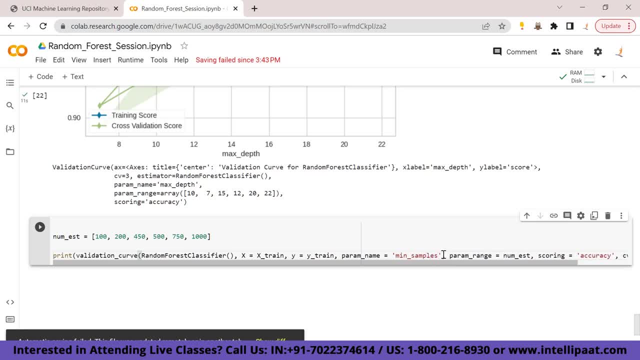 split And we'll change these values Okay, To the number of samples that we want at each split range. So let us say we want three, we want six, we want four, five, eight, 12,, 15, and let's. 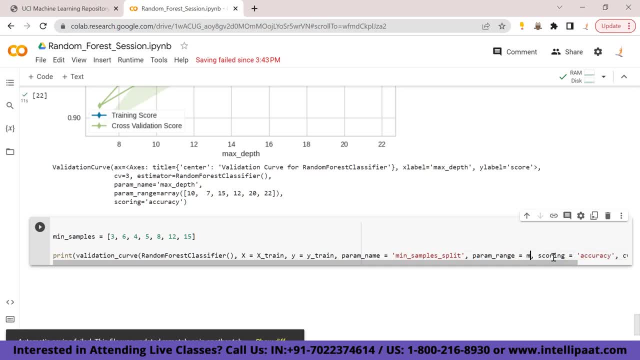 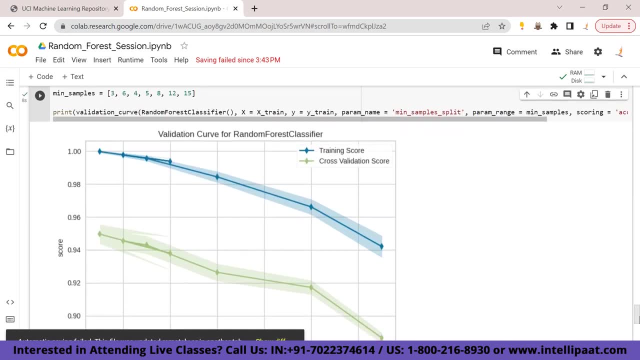 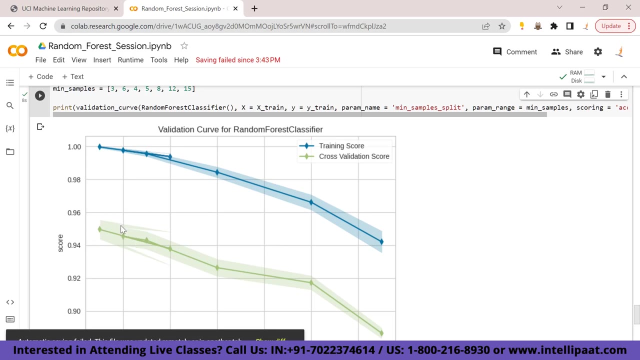 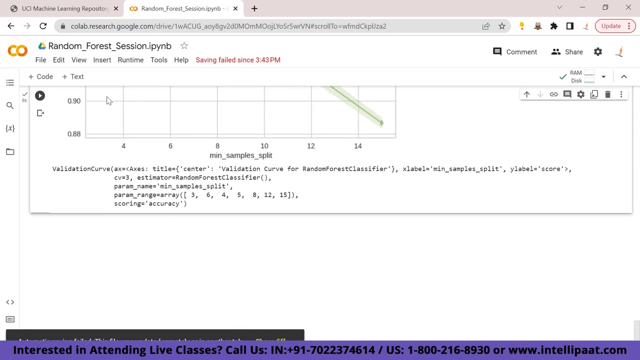 change the name of param range over here. We'll set it to minimum samples, Okay, Okay, And after running this block, you can see that we are getting maximum accuracy when minimum underscore sample split value has been set to three. So what we'll do is we'll create another classifier and we'll pass all these optimized value to. 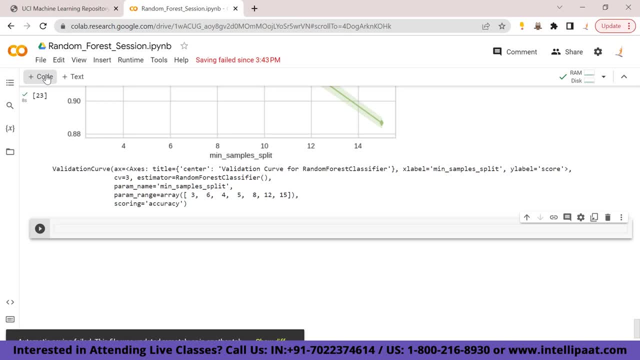 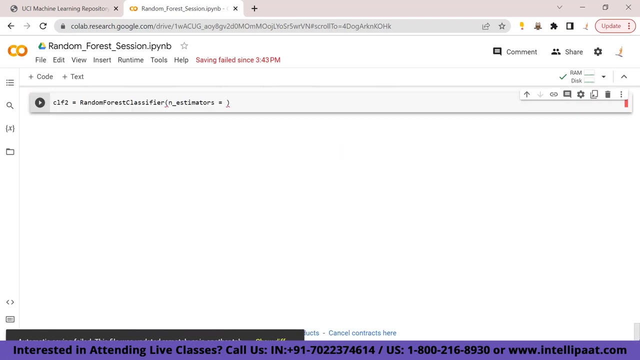 it All right. So let us create the new classifier, CLF two is equal to random. Okay, So random forest classifier and N underscore estimators is going to be thousand. Then minimum underscore samples underscore split is going to be three. 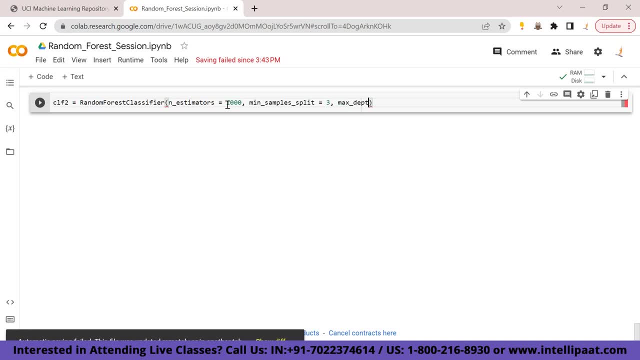 Okay, Okay, So this classifier is going to be three, And then maximum depth is going to be 15.. And we'll set random state at zero. Now let us fit our data to this classifier. Okay, Let's see Okay. 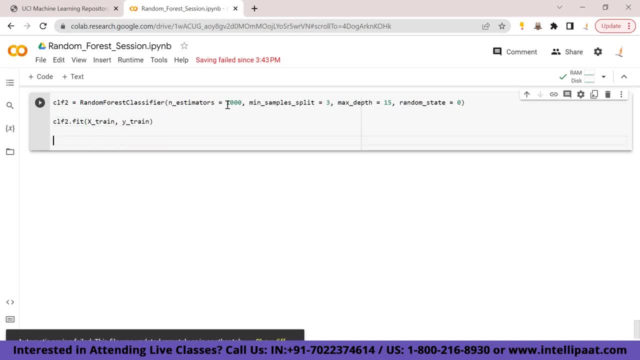 and we'll name predicted variables as pred2 and we'll use clf2 dot predict function over here and inside. it will pass X test and will also print the accuracy score for this particular model, pred2 comma Y underscore test. and here you can see that we are getting ninety. 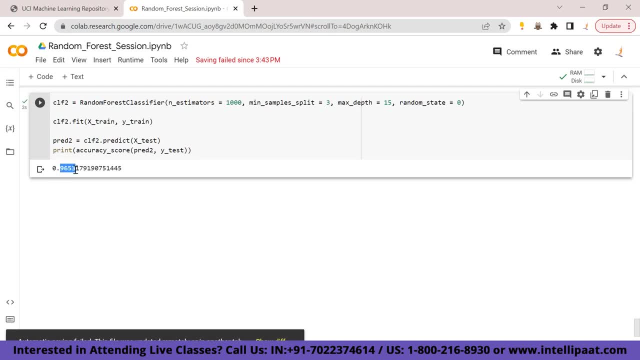 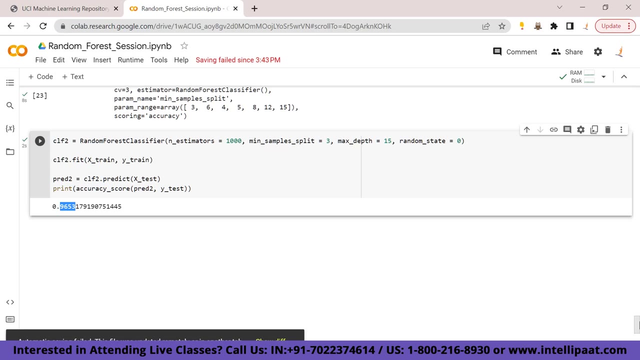 six point five, oh, three percent accuracy, which is almost close to the accuracy that we got previously. now, the accuracy that we are getting over here is called accuracy, and the accuracy that we are getting over here is called is less compared to the accuracy we got for the classifier one which was set to constant. 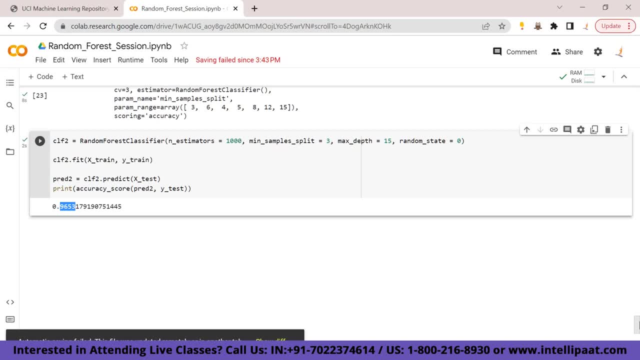 basically The reason behind this is that the other parameters that are left to be tuned are there in this classifier number two. If we optimize them, if we tune them and then add them to this classifier, then definitely we'll get improved accuracy value over here. Okay, the next very 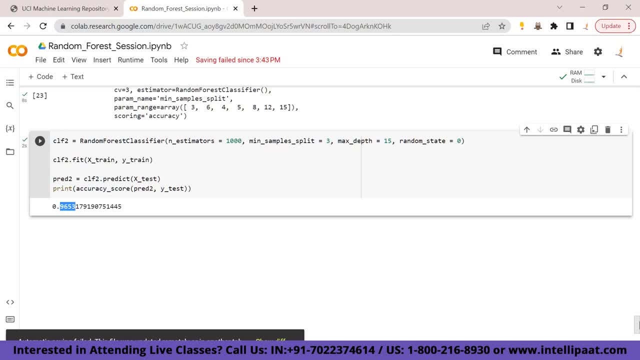 interesting and powerful thing that you should know about random forest is that you can learn the importance of feature with its use. I mean, you can use this algorithm to extract the important features from your data set itself. So let me show you how you can gauge the importance of 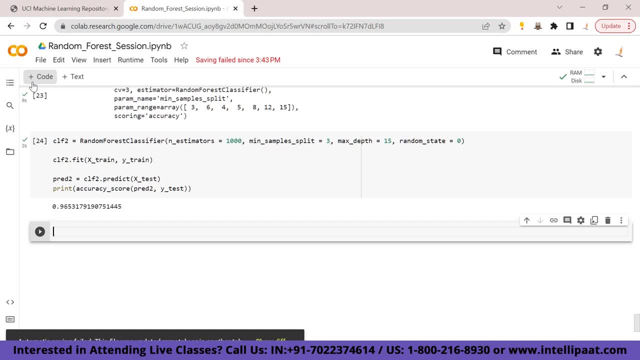 different features available inside your data set using this particular machine learning model. For that purpose, what we are going to do is we are going to use method named as feature underscore- importances, underscore over here- And that will return the importance and percentage for each and every column available inside our data set. So I'll create this pdseries object. 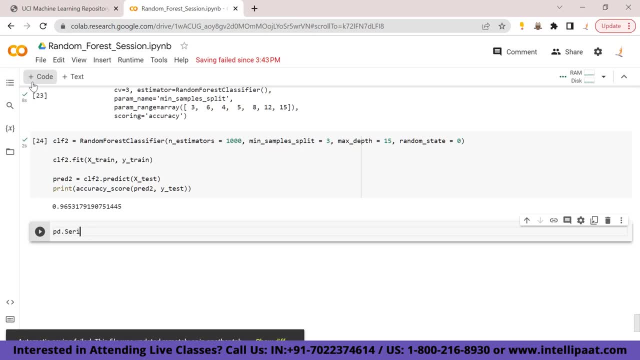 over here And inside it I'll use the important function scores. Now I'll set index as training samples, columns And we'll also sort these values so that we'll get higher score at the top And we'll name this object as feature underscore scores. 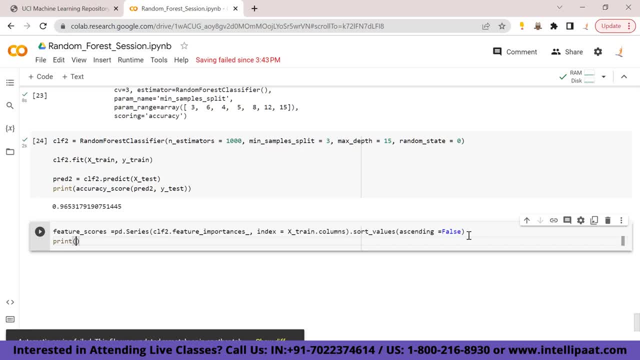 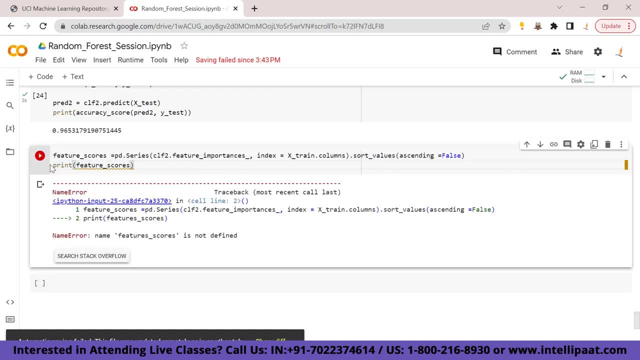 We'll also print these individual scores. Okay, I've made a spelling mistake over here, So I'll rerun this. Okay, here you can see that we are getting this the importance values in percentage over here. Well, let us visualize them with the help of. 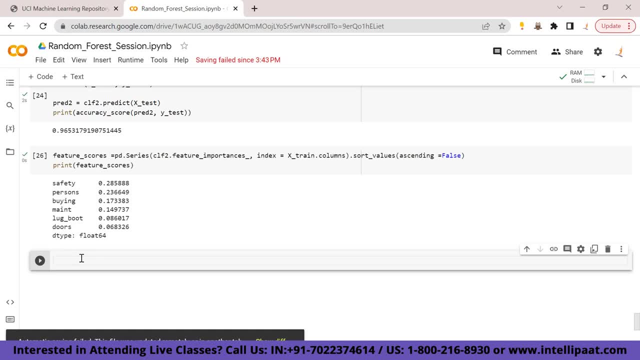 barplot to visualize them better, So I'll use snsbarplot. I'll set x equal to feature scores And I'll set y as feature underscore scores. dot index, which basically is going to be the columns of our extreme sample or our feature names. all right, so I'll set PLT dot X label as. 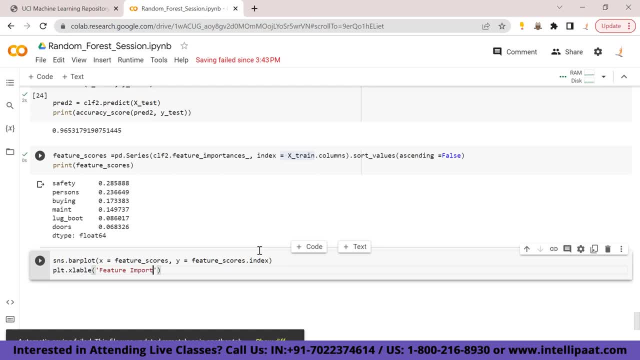 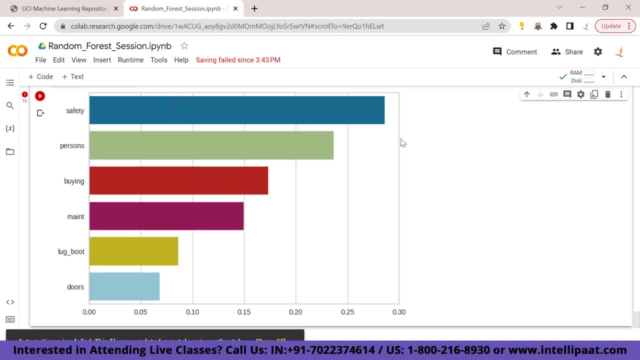 feature importance score. here you can visualize that safety has the most importance in our data set. safety, persons and buying are the top three contributing columns towards the learning of our model. so let us do one thing: we'll remove the two least performing columns from our data set and 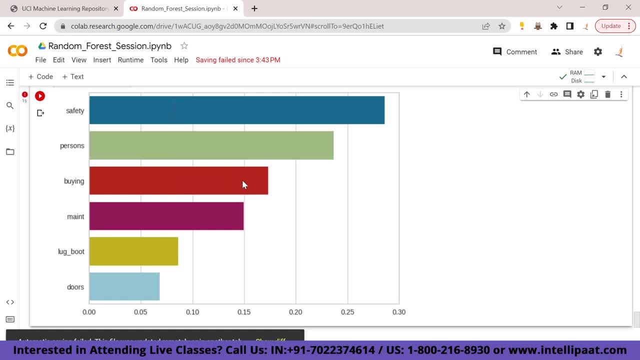 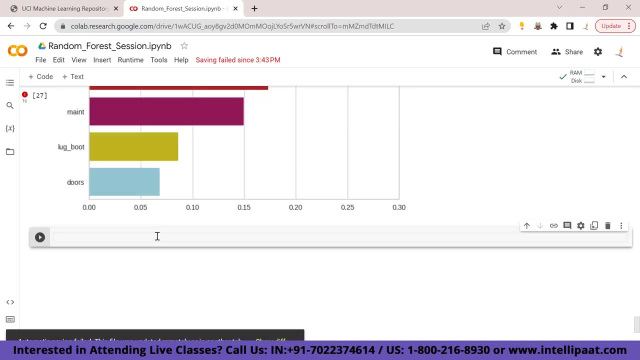 we'll create new classifier and let's see what kind of accuracy the model generates then. so let us create one more classifier. CLF 3 is equal to random forest classifier. now we have to remove these two columns out of our data set, so what we'll do is we'll create the new X. 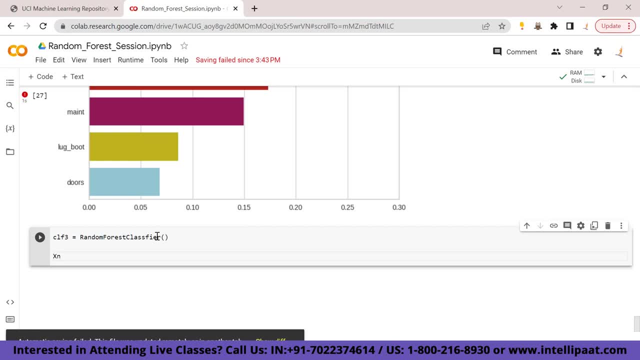 and Y split, so I'll name it as X n. X n will be DF dot. drop column named as to us, then luck, boot and mint, and we'll set access equal to 1, because we want to remove these columns from our data frame and we'll set why you as DF class. 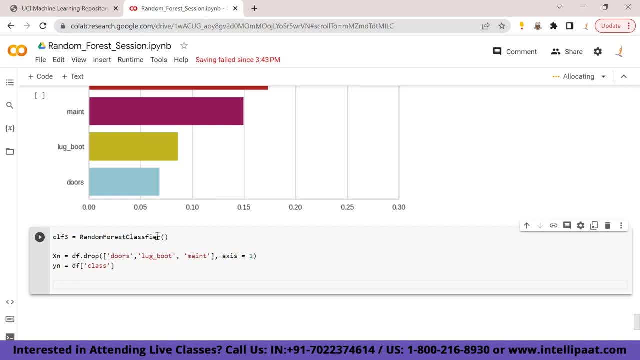 now we'll split our data: X underscore T片, comma X underscore test and comma why protocol train, and comma y underscore test n, and it will be equal to train underscore, test underscore split and inside it will pass x, n, y, n and will set test size equal to 0.3 again. Now we will fit our training data to our model clf 3 dot fit. 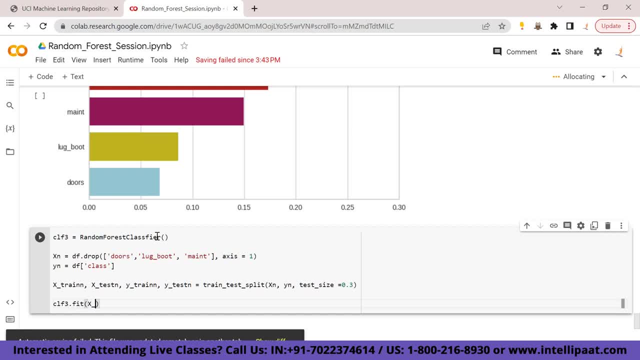 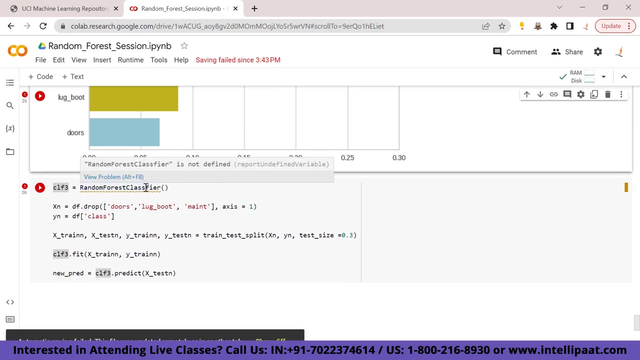 x underscore train n. comma y underscore train n, and we will save predictions inside the model inside variable named as new parade and will set it to clf 3 dot. predict x underscore test n. Now let us run this block. Well, guys, I have made one mistake over here, So the